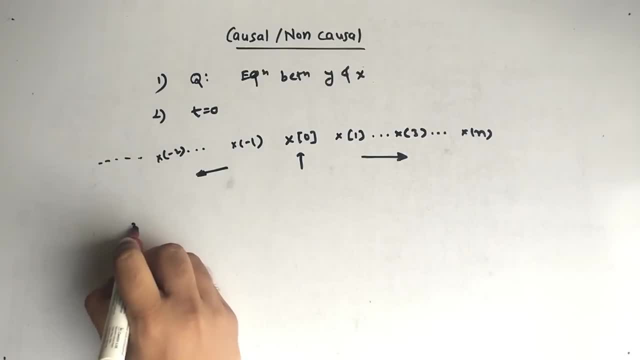 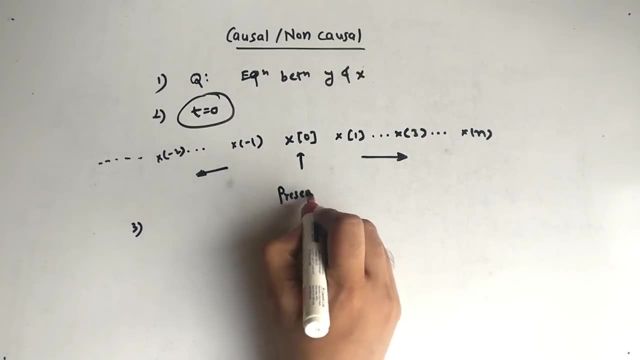 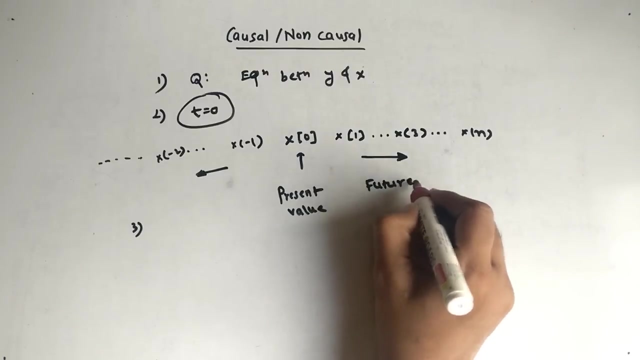 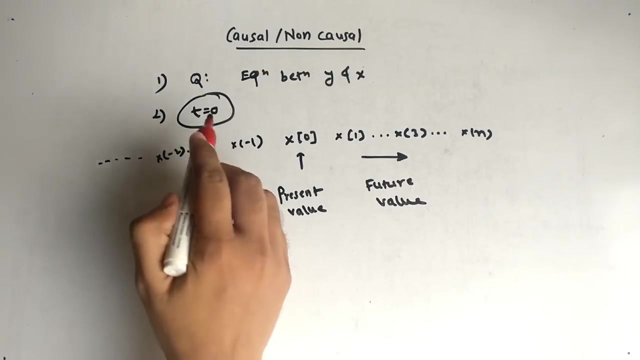 this is important. This arrows means what. So let's see that Whenever you put t equal to 0,, you get present value. Alright, or you can get future value, Or, similarly, you can get past value. So, when you put t equal to 0,, either you can get x of 0 plus, let's say, x of 3, or 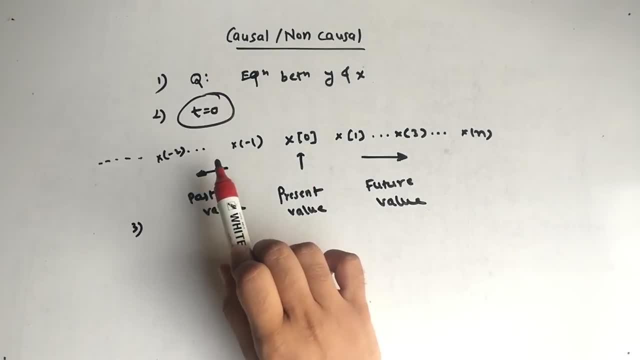 you can get x of 0 plus, say, x of minus 2, like this. So there is combination, Like: whenever you get present value, present and past. whenever you get this combination, this means your system is causal. Okay, now, when you get present and future, this means your system is. 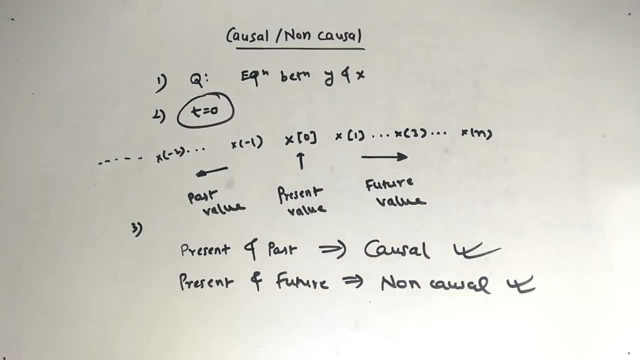 non-causal. So this is very simple. So let's take a recap of the steps. First, the question is in x and y equation. Now put t equal to 0.. After putting t equal to 0, you will get some combination like present value and future value or past value and present value. So let's check: if present and past is the combination, then the answer is causal. If present and future is the combination, then answer is non-causal. 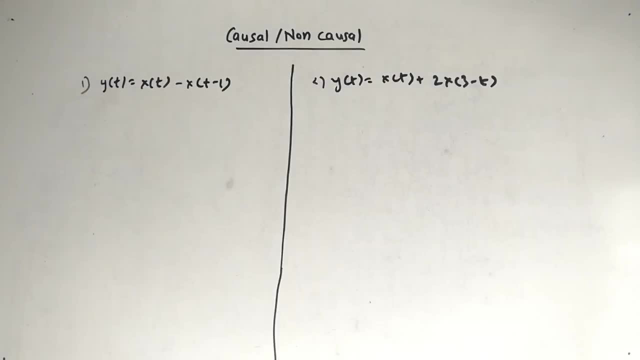 So let's see some examples. So the first question is: y of t equals x of t minus x, of t minus 1.. So the equation is in y and x. Okay, now we have to put t equal to 0. After putting t equal to 0, we get y of 0 and we get x of 0 minus x of 0 minus 1, and this is x of minus 1.. So you can see we are getting. 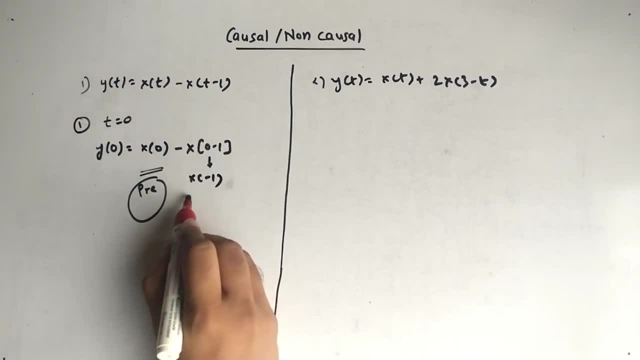 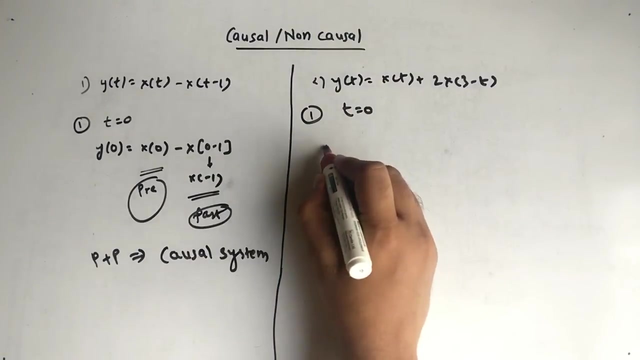 value. okay, we are getting present value and we are getting past value. so what is this combination? so present plus past? this is causal system, okay. so let's see the second question. again, we put t equal to 0. after putting t equal to 0, we get y of 0, that is equal to. 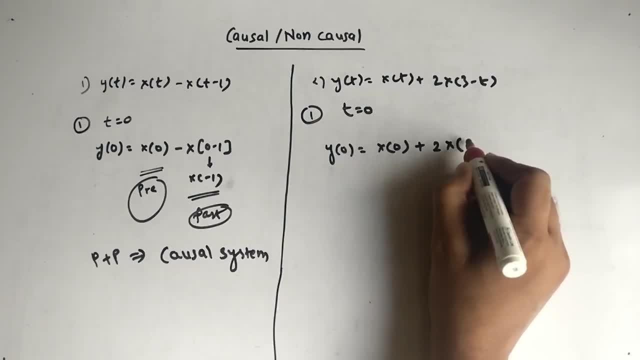 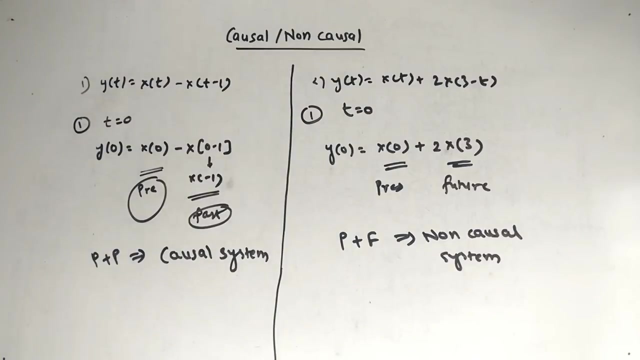 x of 0 plus 2 times x of 3, because 3 minus 0 is 3. so you can see here again, we get present and we get future. so what is this combination present plus future? this is non-causal. so I hope you are getting the steps and how to identify whether it is causal or non-causal. 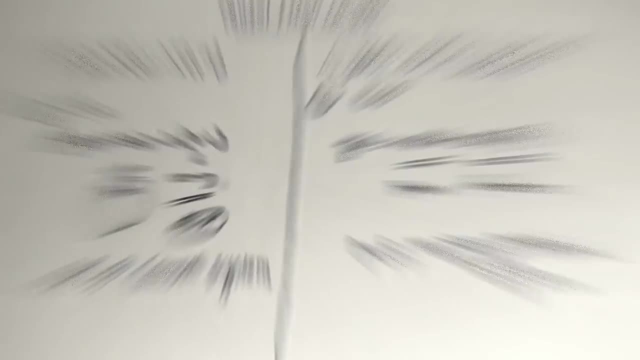 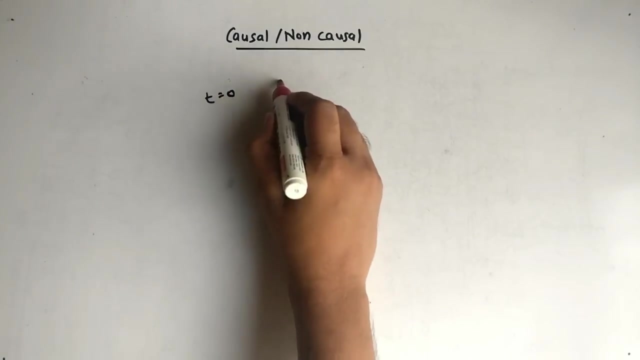 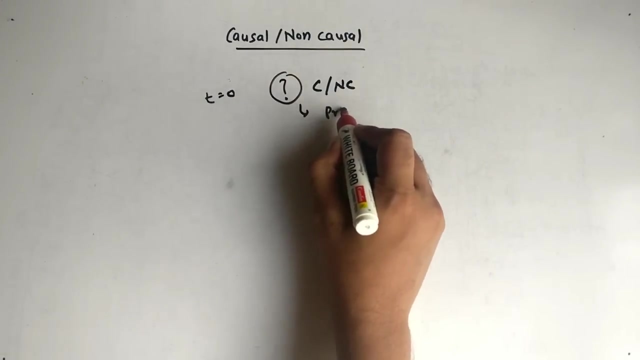 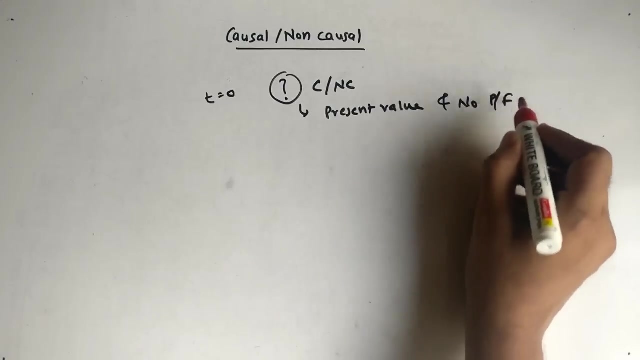 let's see some interesting example as well. now my question is: what if we put t equal to 0 but we are still confused whether it is causal or non-causal. why we are confused? because it only shows present value and there is no and no past or future. when we put t equal to 0, then what we have to do? so let's take 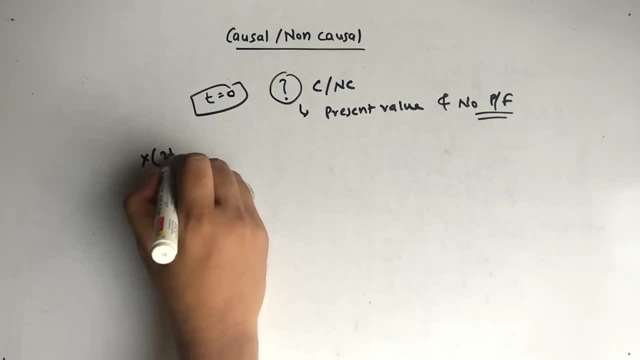 that example. so our example is x of 2t. suppose we have x of 2t. now put t equal to 0, let's say y of t equal to x of 2t. after putting t equal to 0, we get y of 0, that is equal to x of 0. so now we are confused. what? 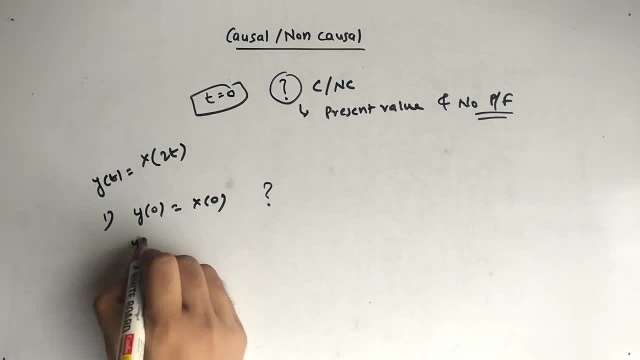 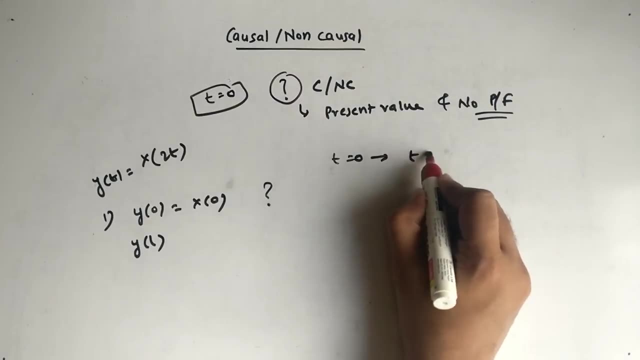 is this. then take another value. let's put y of 1. this means we are putting, after we put t equal to 0, we are shifting to t equal to 1. so let's check at t equal to 1 is it same like we get x of 2t. 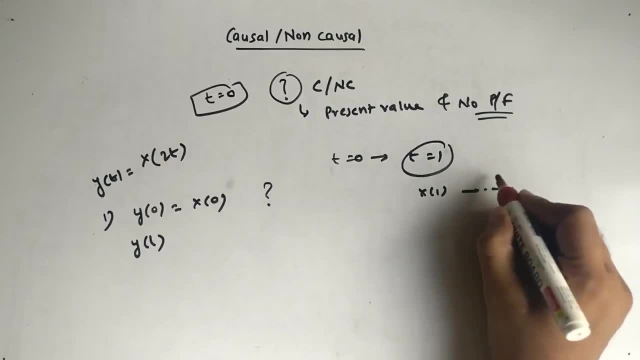 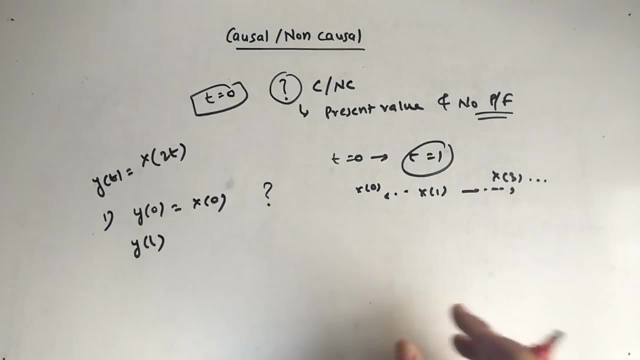 or we get x of 1, or we get x of this future value, that is, let's say, x of 3 or something, or we get past value, let's say x of 0 or something. we have to decide this by putting t equal to 1. so after putting t equal to 1, we get x of 2. now you can see, we started at x equal. 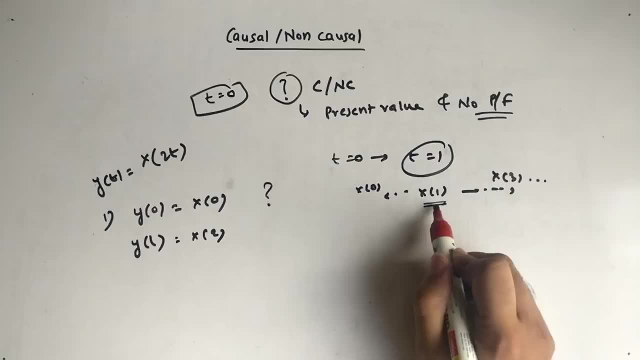 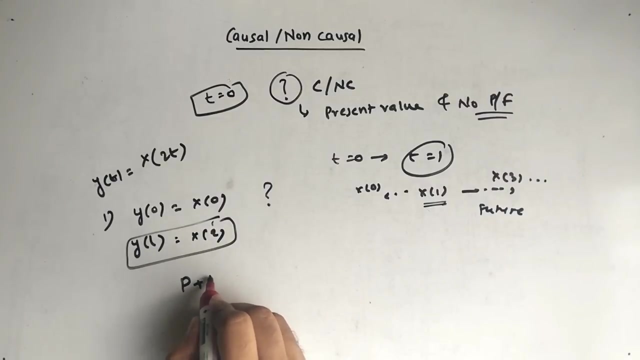 to t equal to 1, so x of 1 is here. but now you can see where is x. x is 2, so it is in future. so what does this mean? this means that it depends on present plus its value is future. so present plus future is non-causal. let's take another example, suppose, suppose i have 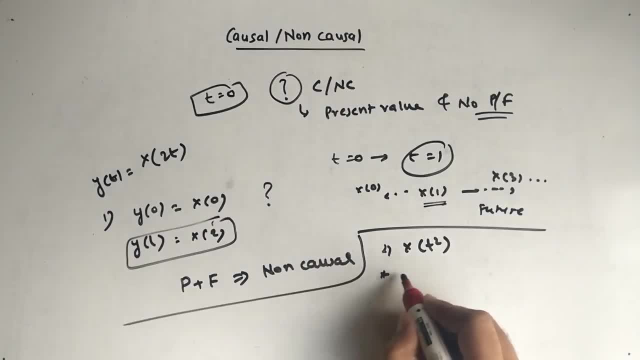 x of t square. now what again? x of t square equal to y of t. so at x. sorry that t equal to 0. so y of 0 equal to x of 0 again. same condition now. what is this answer? so now put t equal to 1. when we put t equal to 1 again, we get same again. there is a confusion. 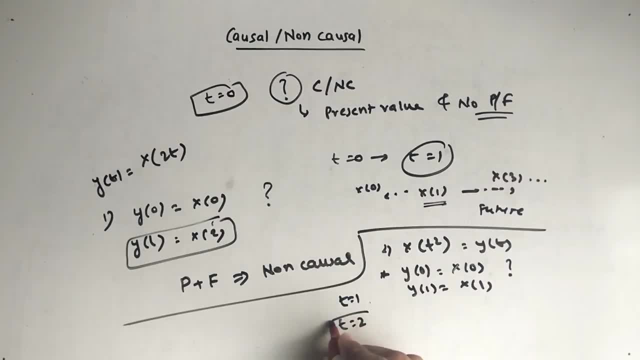 what is the answer? now put t equal to 2. so whenever you fail to get an answer- and let's say t equal to 0, you fail to identify whether it is future or past. go for t equal to 1. now again you fail to identify. then go for t equal to 2, and so on. alright, so when you put t equal, 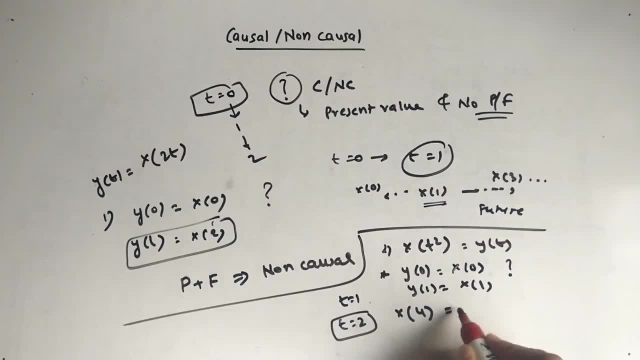 to 2. now you get the answer x of 4 and y of 2. now you can see. now it depends on future. so again, past plus future is non-causal. so both the system, this and this, both the system, are non-causal system. 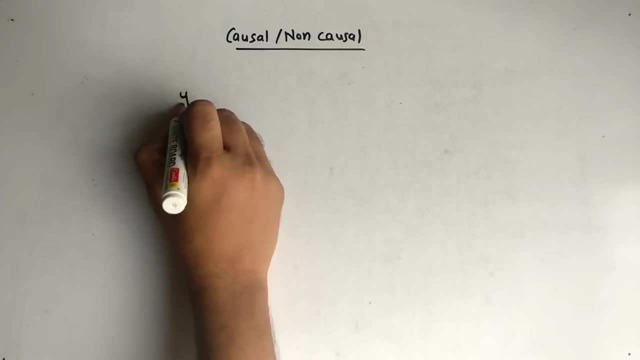 now this example is very interesting. the example is very interesting. the example is y of t equal to t times x of t. so what is this system? let's take whether it is causal or non-causal. so first step was put t equal to 0, so we get y of 0 equal to. 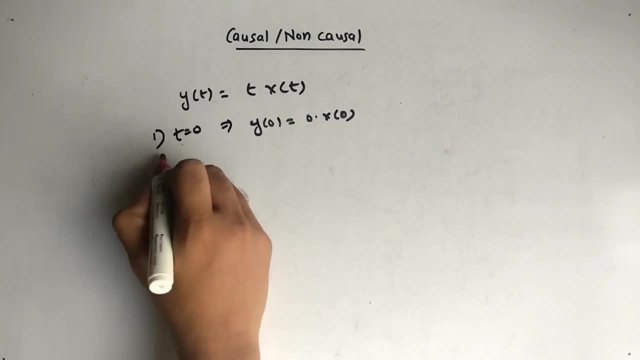 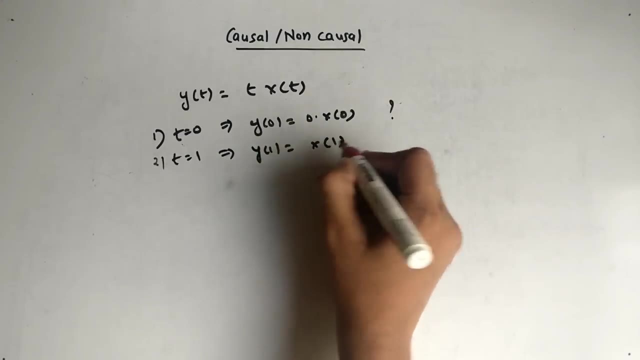 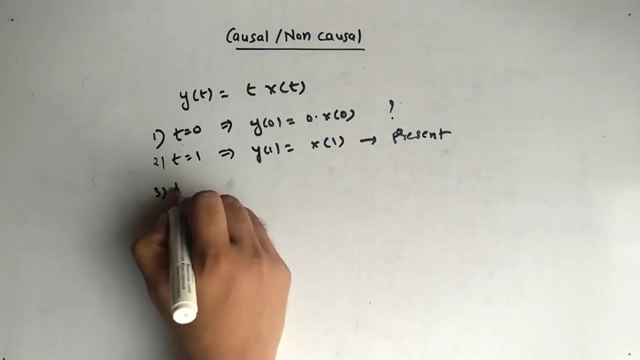 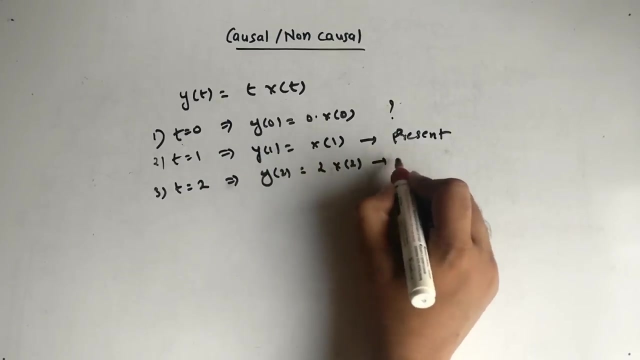 0 times x of 0. okay, then we have to put t equal to 1, because we are still unsure. then y of 1 equal to x of 1. okay, at this we get present value. we get present now. at t equal to 2, again, we get y of 2 equal to 2 times x of 2, again present. 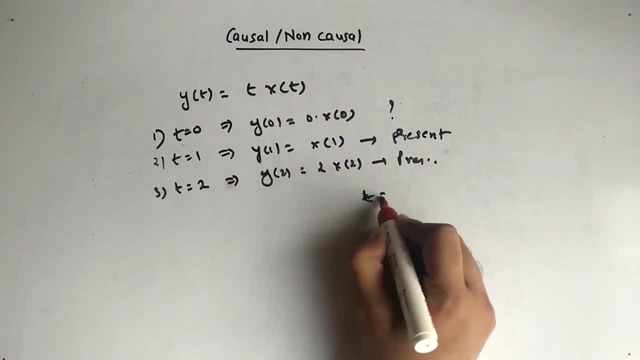 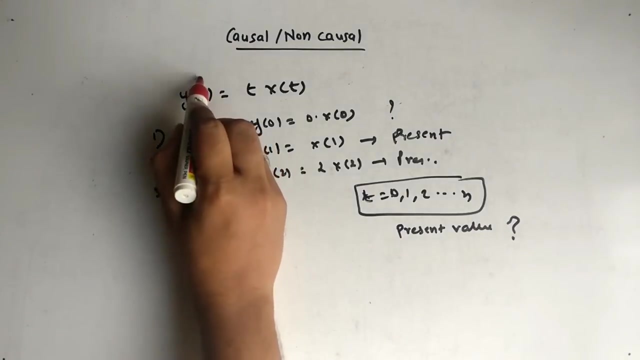 now the problem here is: you put t equal to 0, 1, 2 or n. the problem here is: whatever value you put, you will get same, like you will always get the present value. why? the question is why? because these two function: y of t and x of t. 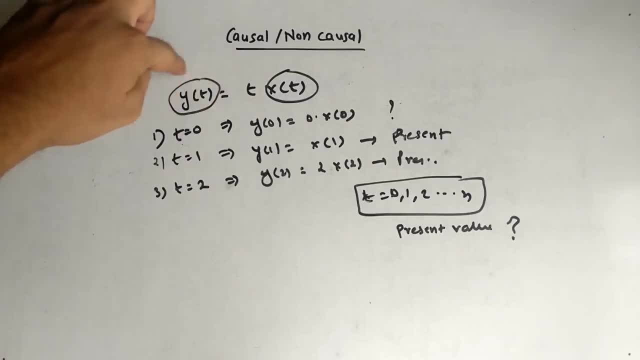 they will never change. like at 1, both are 1, at 2, both are 2. so this will never change. so now we have to put some interesting thing, and that is, if you put negative value again, we will get the same. so minus times x of minus 1. so the problem here is at negative value. 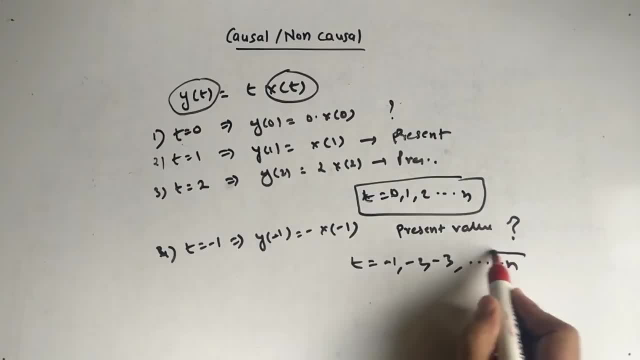 also, let's say minus 3, and so on, minus n, let's say minus 3, and so on, minus n, we will get present value. so now, what to do? okay, so now you have to understand that if there is only present value, only present, alright, only present, then the system is causal system. 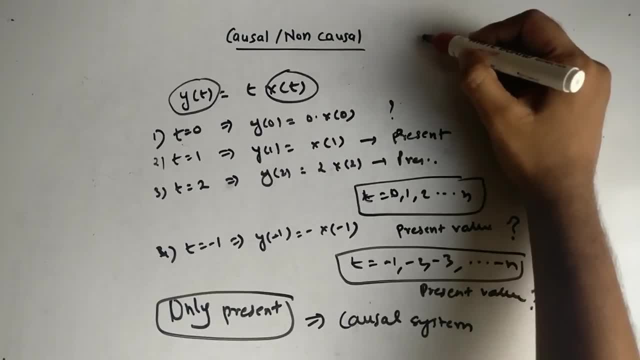 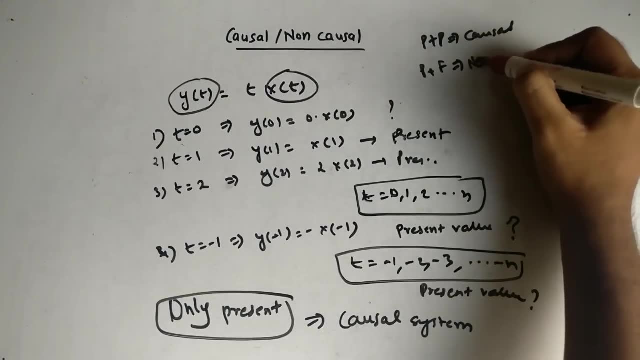 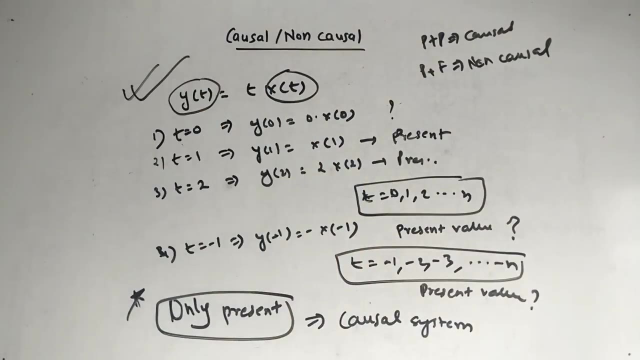 so this was very important. like you know that, if this system is present plus past, then it is causal. Okay, If the system is present plus future, then it is non causal. this you know, but this is the unique case and therefore this function is very important. in this function, we get 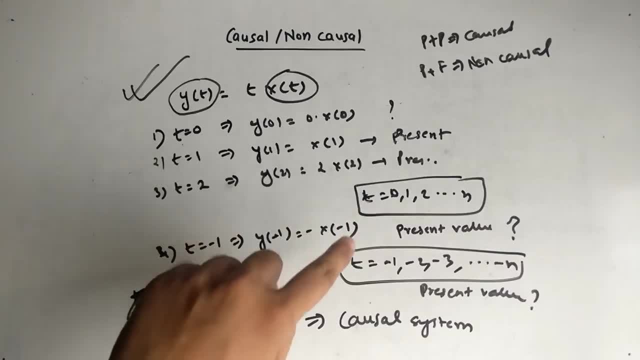 only present system. you put any value, any positive value or any negative value, you will get the same, that is, the present values. at that time there will be no past or there will be no future. so if the system has only present value, then it is a causal system. 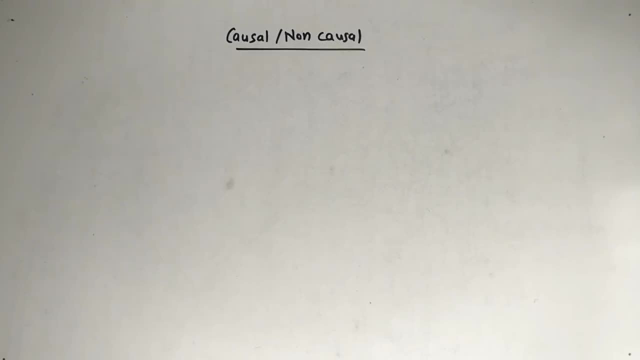 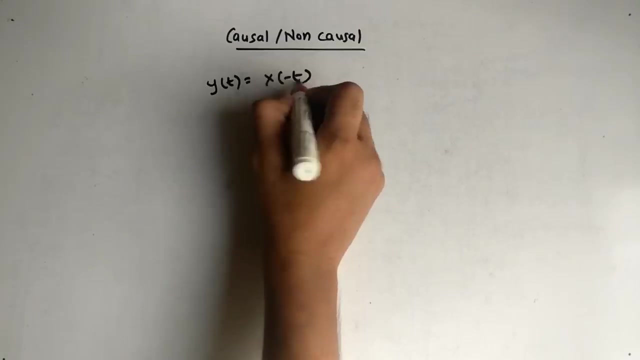 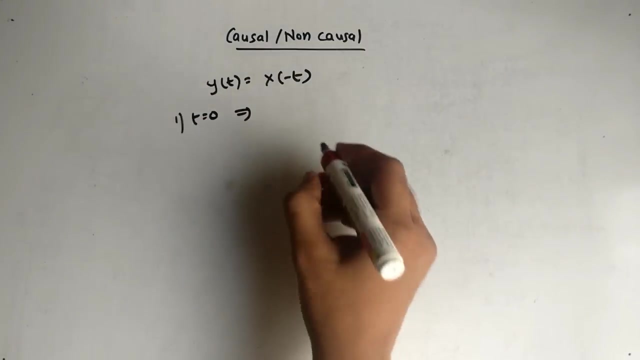 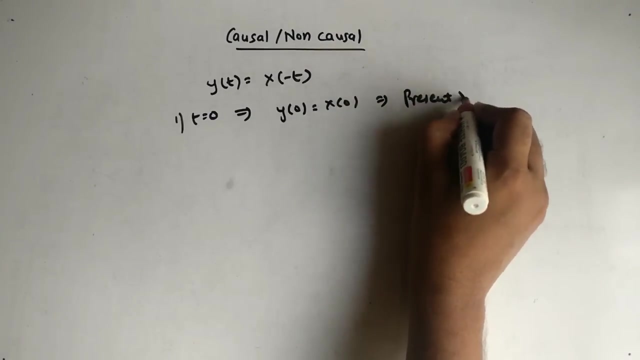 There is one more unique function. so let's see that, suppose I have this: y of t is equal to x of minus t. so now what again? you have to put this: that t equal to 0, t equal to 0, we get y of 0 that is equal to x of 0. okay, in this condition we get present value present. 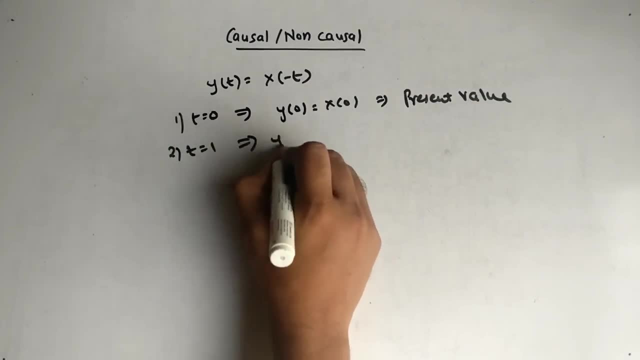 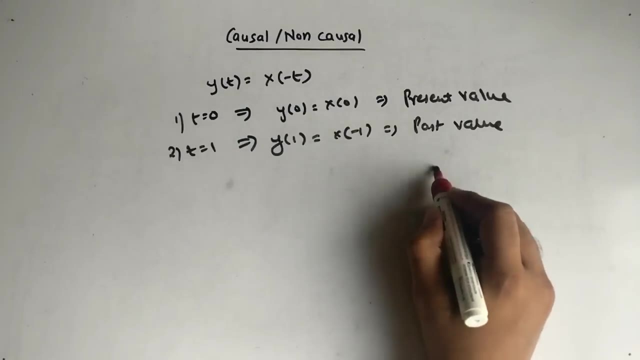 value. Now, If t equal to 1.. We get y of 1.. Okay, So t equal to x of minus 1, so here we can get past value. okay, so we have this two condition present plus past. so you are thinking the answer would be causal, alright, so if you are, 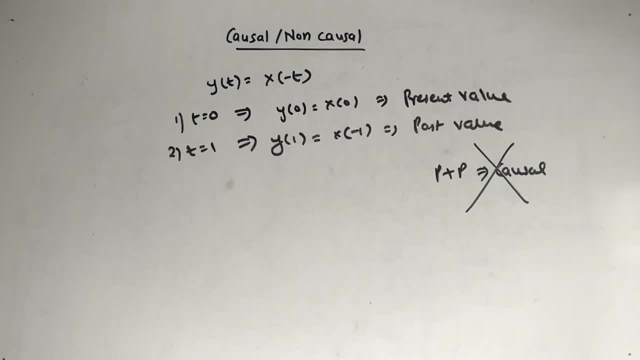 thinking the answer is causal. you are wrong. why? because in last example we checked for t equal to 0. alright, we checked for t equal to 1 and so on. and we also checked for t equal to, let's say, t equal to minus 1, minus 2, and so on. so we have to check this condition also. 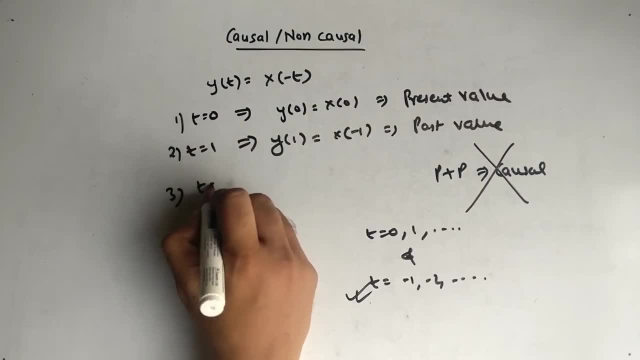 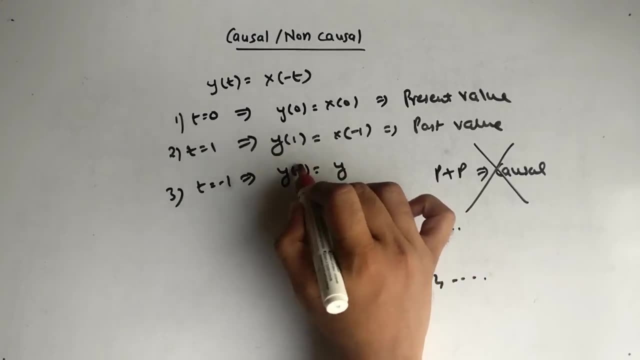 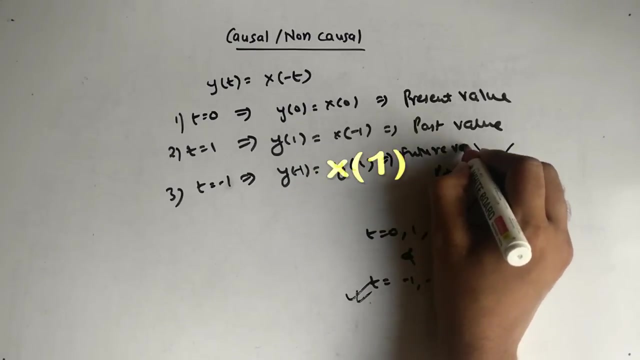 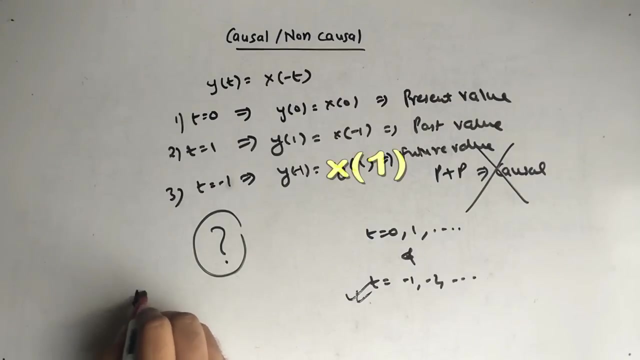 So this condition is: if t equal to minus 1, so answer is y of 1 comma, y of sorry, y of minus 1 and that is equal to y of 1. so this means it is a future value. so now, what is this? again one big question mark. so now, what is this? so this means that all states are: 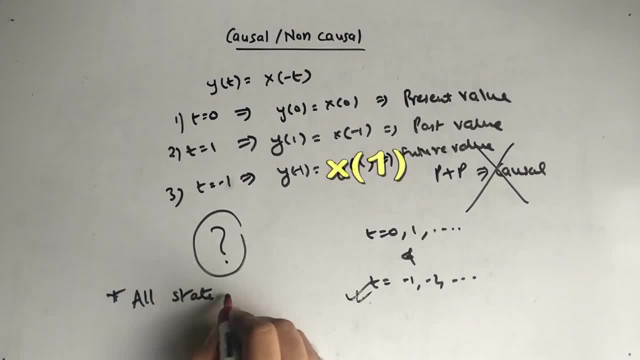 present. alright, let's say all state are present, all state present. All state present means both are present, plus past, plus future, all are present. so now, what will be the system? so the answer for this is: it is a non causal system, and remember this: wherever you see, past value is present by plugging any values, like always. 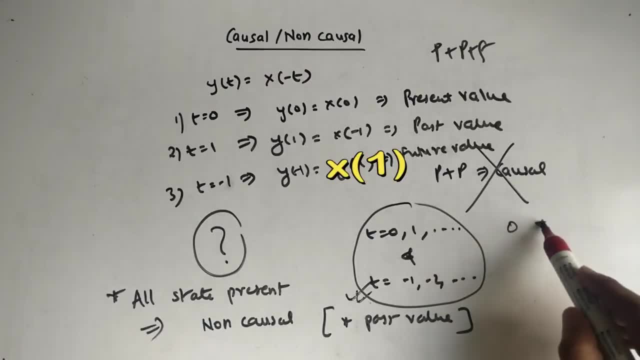 plug the three values: 0 positive value, let's say 1, 2, 3, so on. The negative value, that is minus 1, minus 2, minus 3, and so on. so this three 0 positive values and negative values. you should check for all this and whenever you see that it. 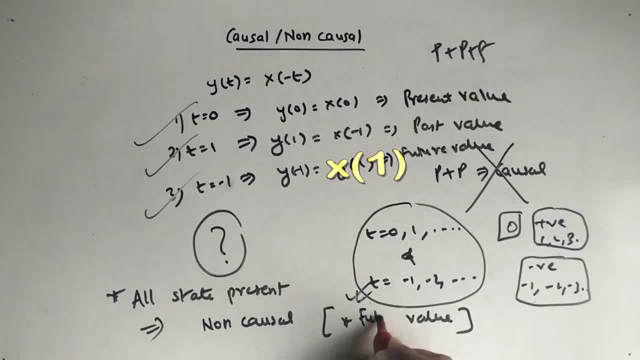 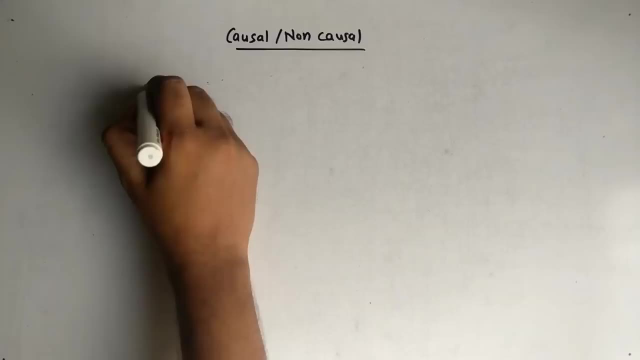 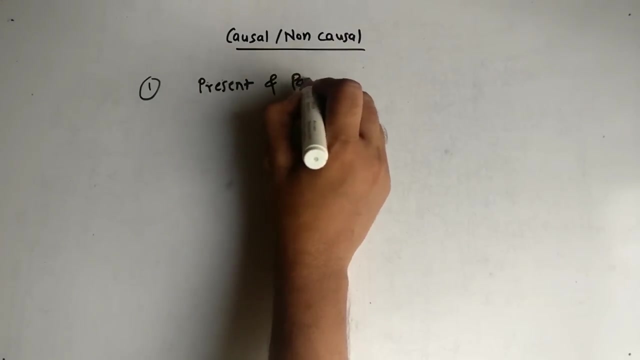 depends on- sorry, whenever you see it depends on future, future value, wherever you see this future value. this means that it is a non causal system. that's very important, so let's sum up everything. So first we sum up this: that whenever you see present and past, you say it is a causal. 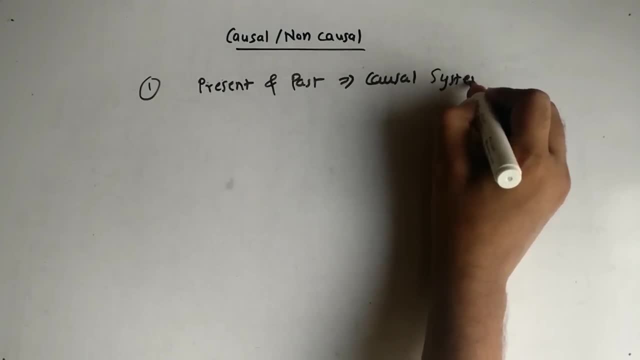 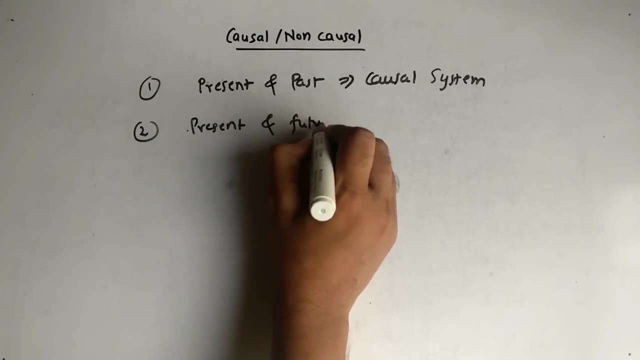 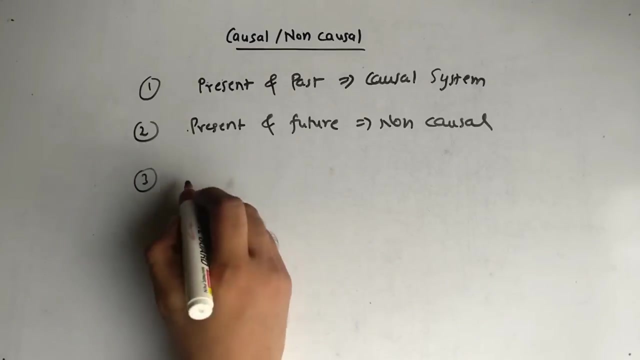 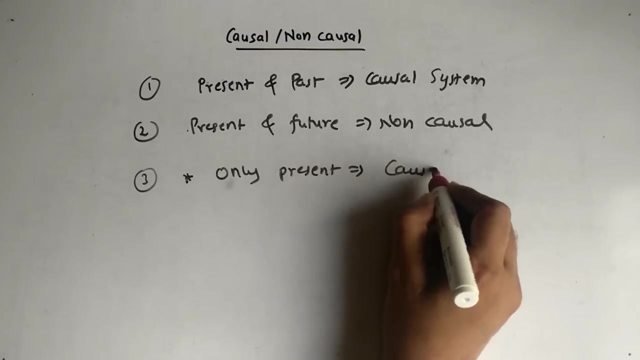 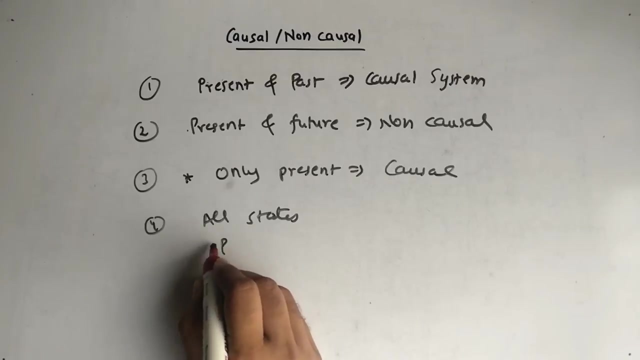 system alright. second we did was: whenever you see present and future, it is non causal system alright. now the unique cases let's take: when it is only present, Only present was, it is causal. and fourth was all states. all state means present, past and future. if all three are present, then it is a non causal. because of this, whenever you 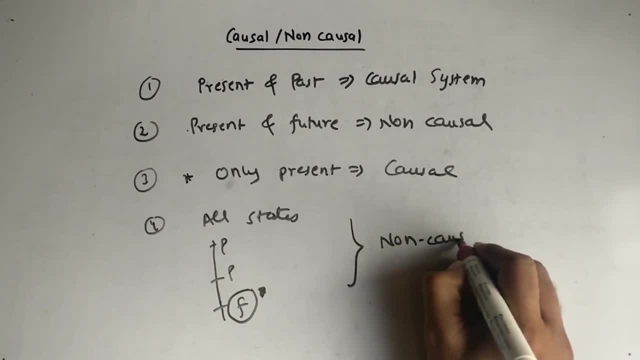 see a future value, then it is a non causal. so basically, these four are the types and these two were the unique functions. So now let's see the non causal. So basically, this four are the types and these two were the unique functions. So now let's see the non causal. 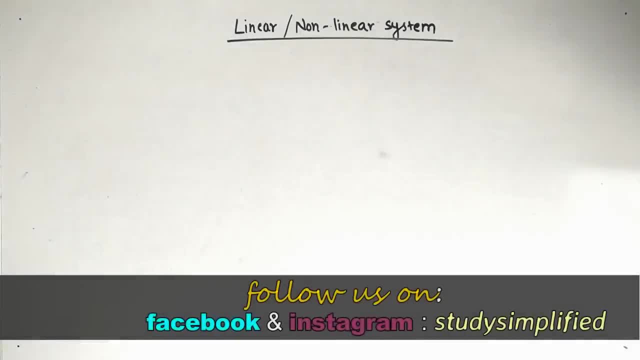 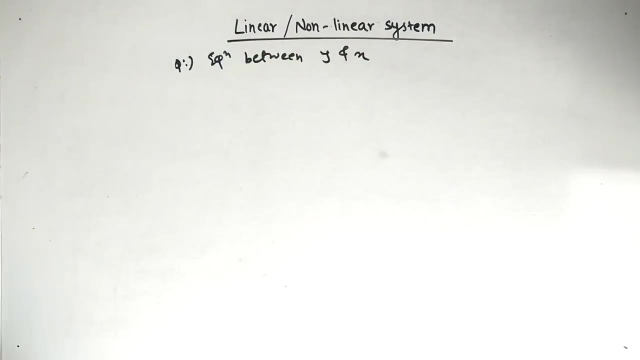 So I hope you got this, Friends. today our topic is how to determine whether a system is a linear or a non linear system. So we have a question, and the question is: equation between y and x. ok, so first step we have to do is find for x1 of t as input, alright, for x1 of t as input, what is y1 of? 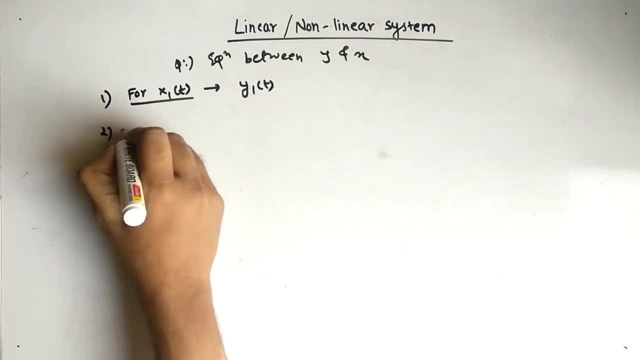 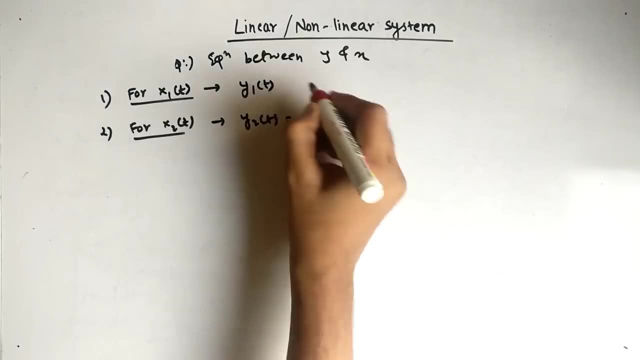 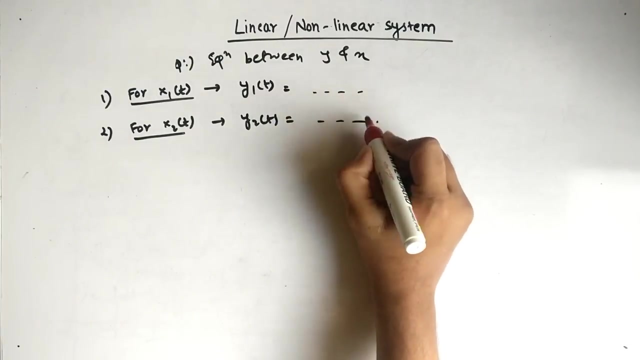 t. Similarly for x2 of t as input. what is y2 of t as output like? because there is an equation between y and x. there would be answer over here in terms of x1 of t and here in terms of x2 of t. ok, 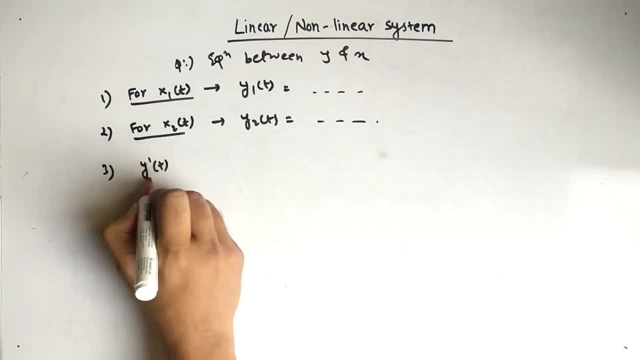 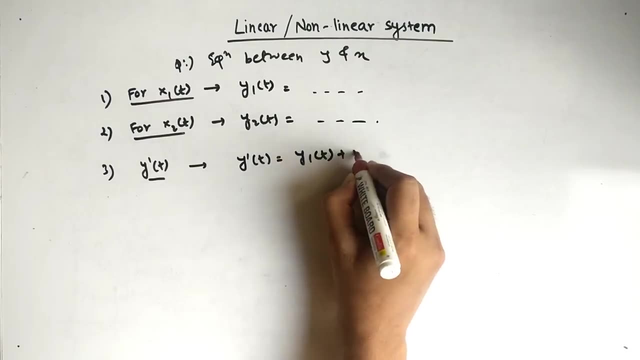 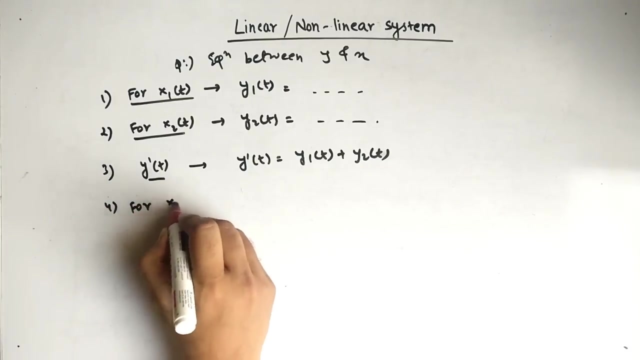 So the third step we have to do is find y dash of t. so now, what is y dash of t? y dash of t is equal to y1 of t, So what is y dash of t? So what is y dash of t? y1 of t plus y2 of t. Now the fourth point. For x1 of t plus x2 of t as input, what is? 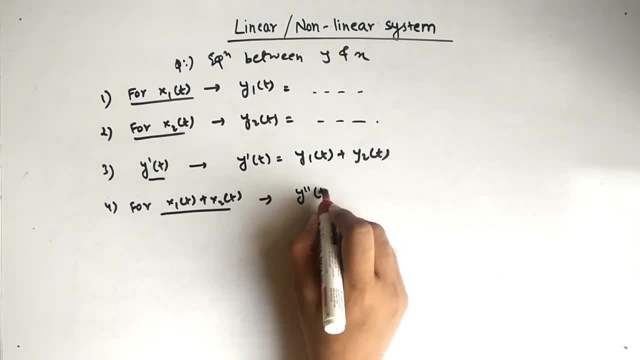 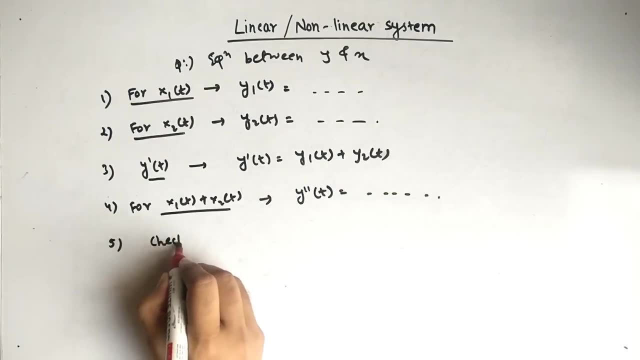 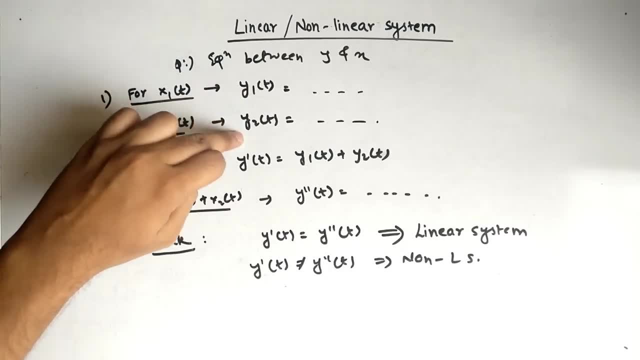 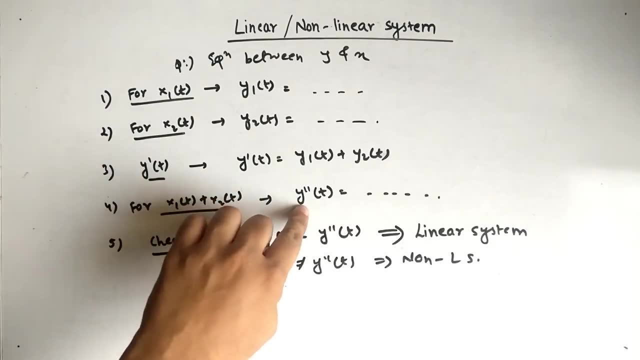 What is y2 of t? Then we have to add both, this y1 of t plus y2 of t, to get y dash of t. Now we have y dash of t. Now we have to find y double dash of t. So for y double dash, 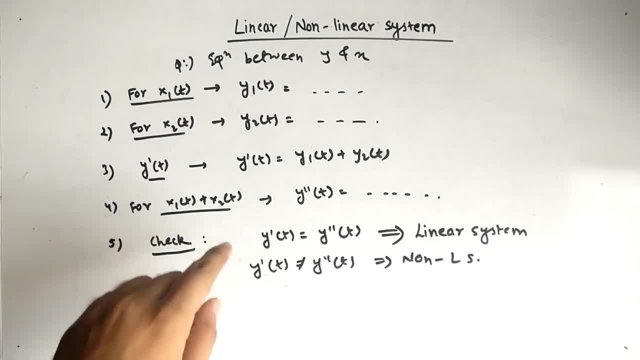 of t. the input is x1 of t plus x2 of t, And then we have to check both y dash of t and y double dash of t. If both are equal, then it is a linear system. If both are not equal, 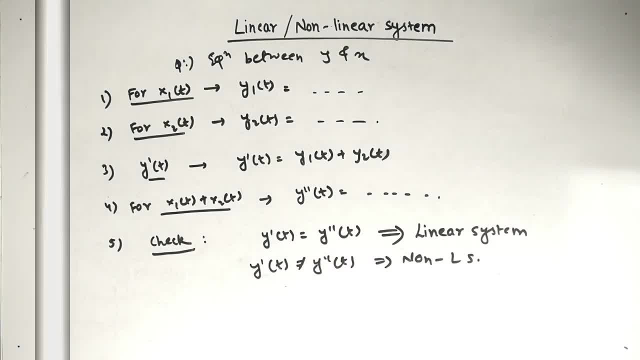 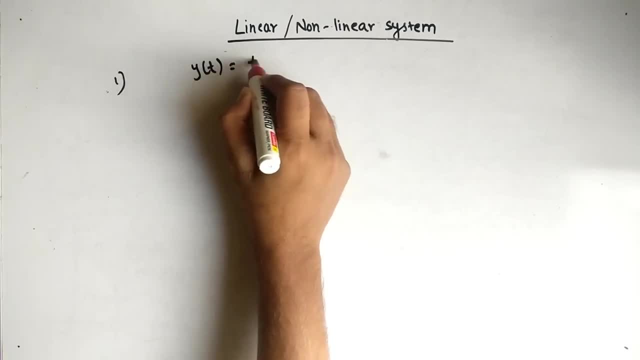 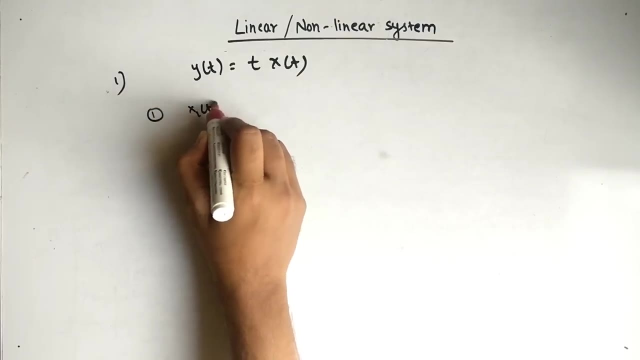 then it is a non-linear system. So let's see an example. So our first example is: y of t is equal to t times x of t. So first step is x1 of t as input. Then what is the output? y1 of t is t times x1 of t. Fair enough. Now, taking x2 of t as input, again y2 of t. 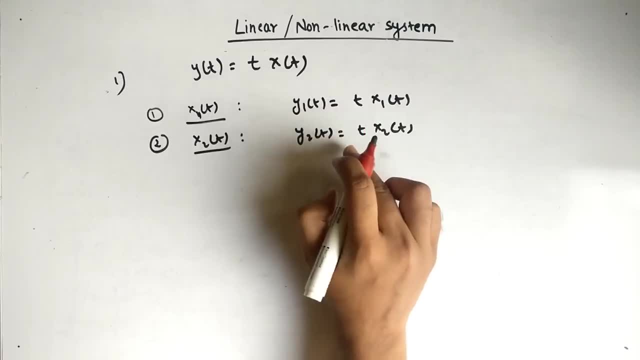 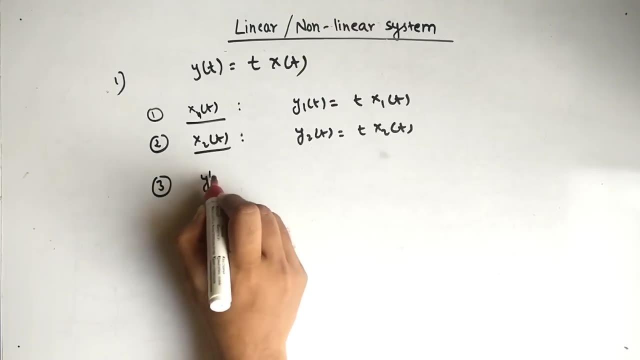 is equal to t times x2 of t. This remains same t, and only the function of y2 of t changes to x1 of t. Simple. Now third step. Third step is y dash of t. y dash of t is what? 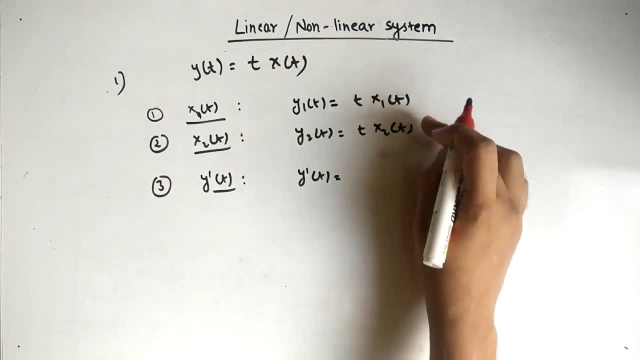 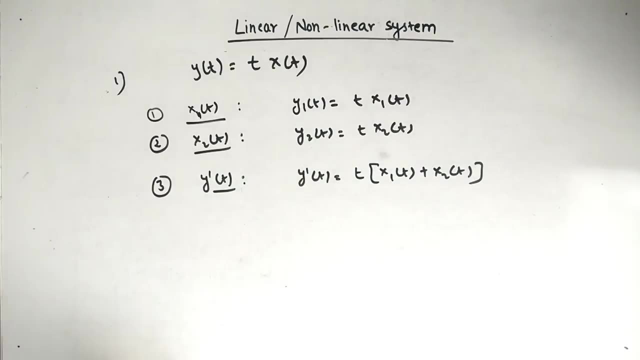 y dash of t is y1 of t plus y2 of t. This means adding these two: Okay, Now t is common: x1 of t plus x2 of t. Now the fourth step Input is x1 of t plus x2 of t. Okay, These. 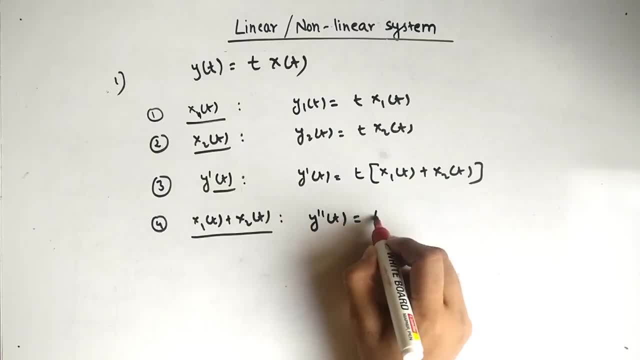 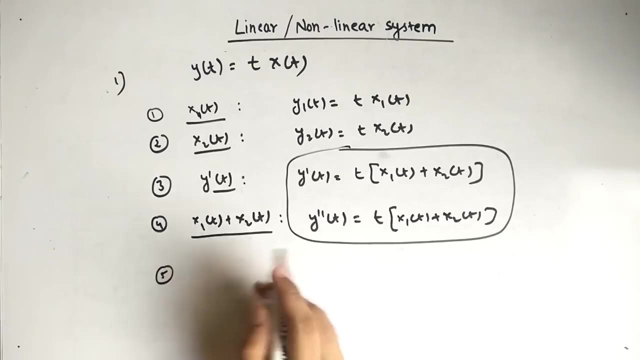 are our inputs. So what is now y double dash of t? t remains as it is. Now x of t changes to x1 of t plus x2 of t. Now you can see these. both Are they equal? Let's check. Yes, Both are equal. So y dash of t is equal to y double. 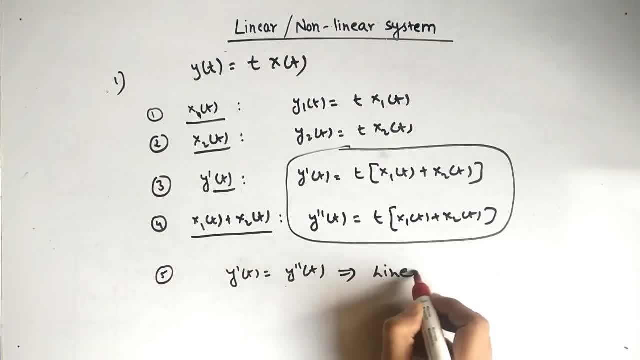 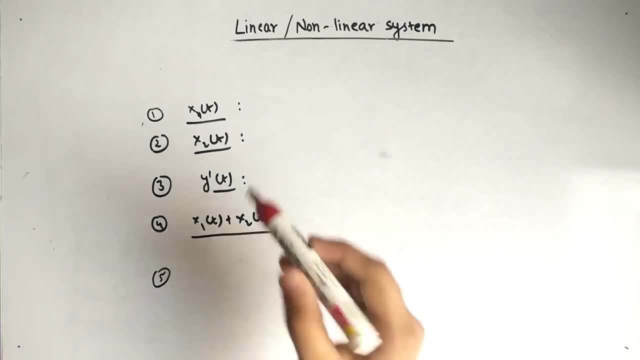 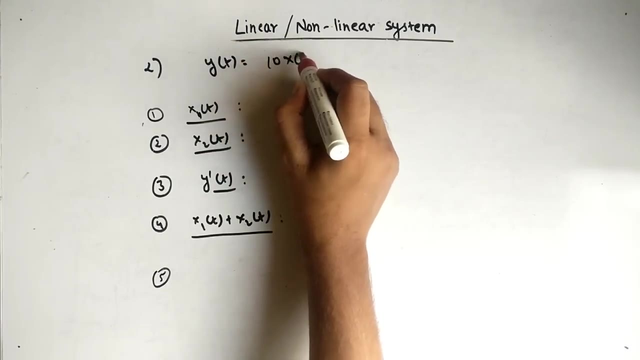 dash of t. This means system is linear. Now let's take one more example. Now the second step: y of t is equal to 10 times x of t plus 5.. So what is the first step? x1 of t as input, So y1 of t is our output, and that is equal to 10 times x1 of t plus 5.. Similarly, 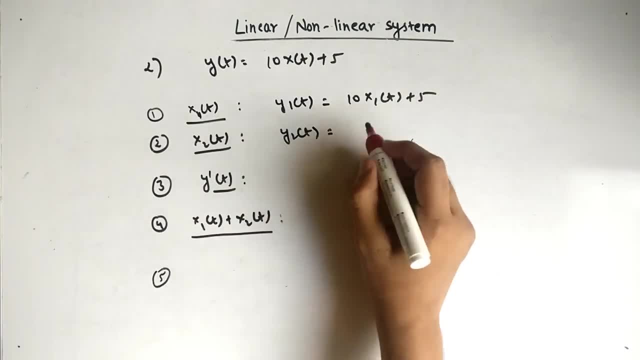 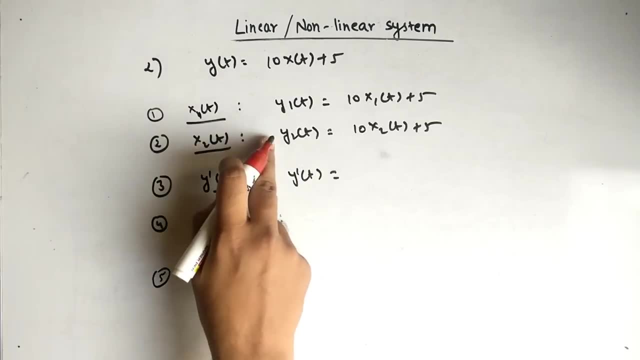 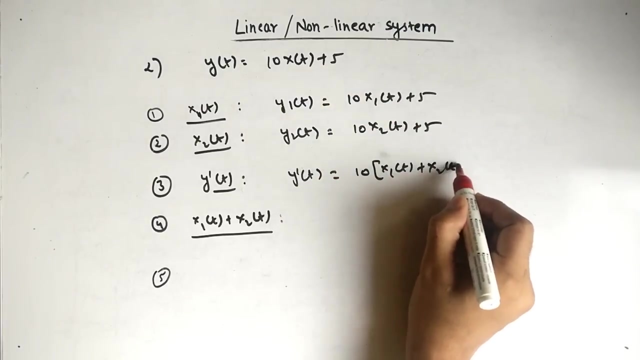 y2 of t is our output and x2 of t is our input. So 10 times x2 of t plus 5.. Now y dash of t was adding both. If we add both we get 10 as common and these two inside the bracket. Okay, But these two. 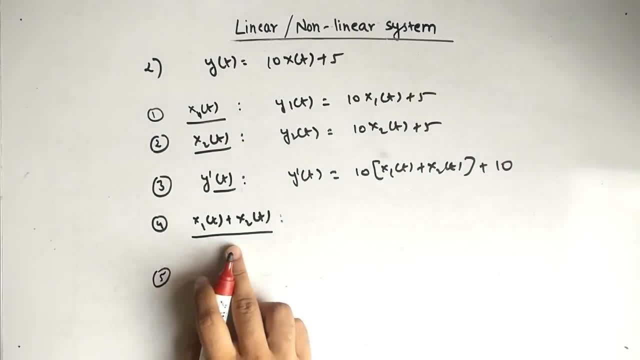 gets add again. So we get 10 here Talking about this y double dash of t as our output. and input is this Now changing x of t to x1 of t plus x2 of t, So again 10 as the multiplying. 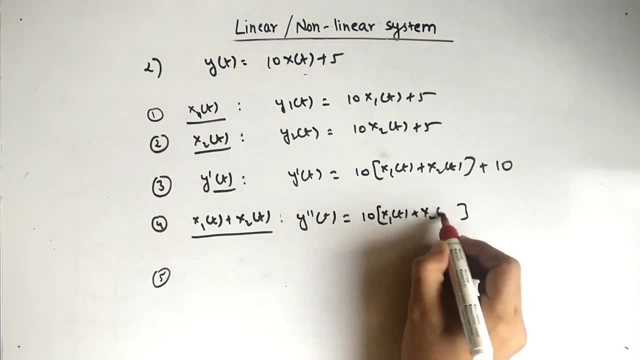 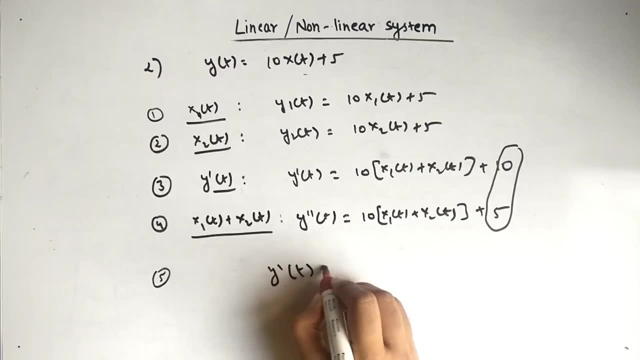 factor and inside the bracket we have x1 of t plus x2 of t, But now we have only plus 5.. So you can see the difference. So y dash of t is not equal to y double dash of t. This means system is non-linear system. 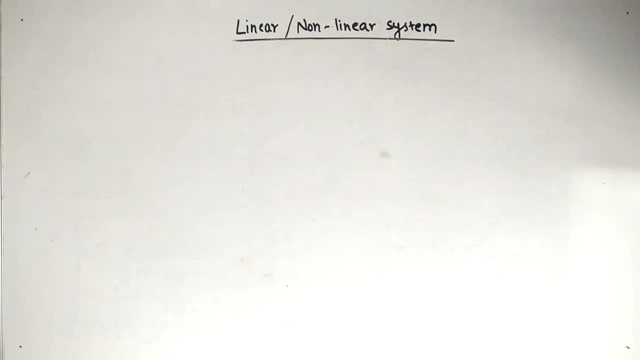 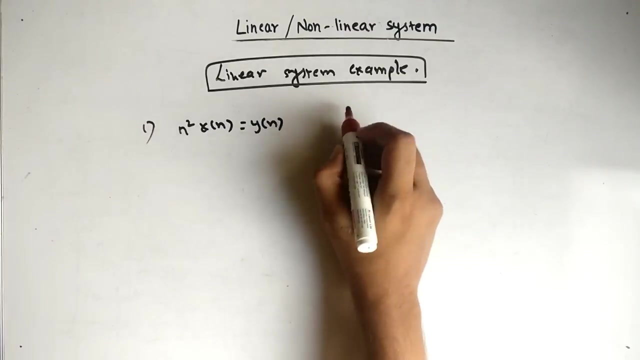 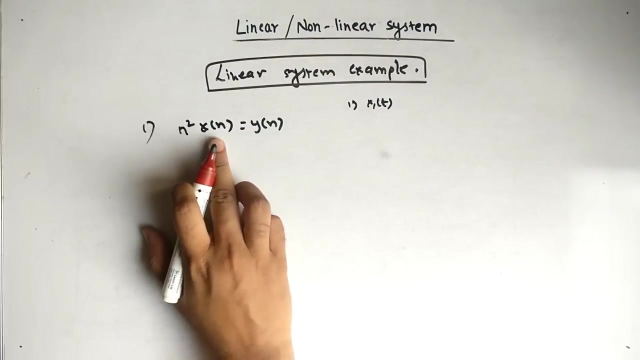 Okay, Now let's see some of the example that comes under linear system. So linear system example. So first example is n square x of n, That is equal to y of n. Now let's Already telescopes. so first we have x1 of t as input. t was for the continuous time. So if we change t to 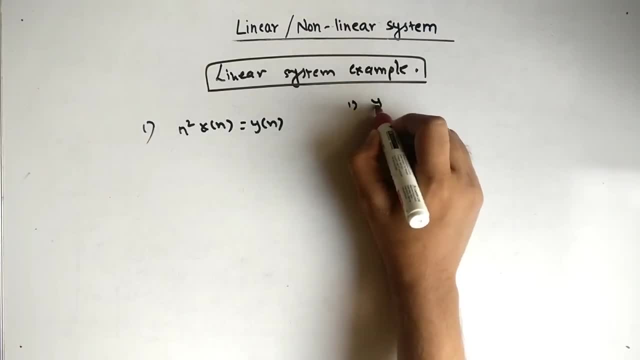 n. then we get discrete time, Alright. So now we are y1 of n, That is equal to n square x1 of n. Alright. Then y2 of n, That is equal to n square x2 of n. So again, y2 of n. Next we have y2 of. 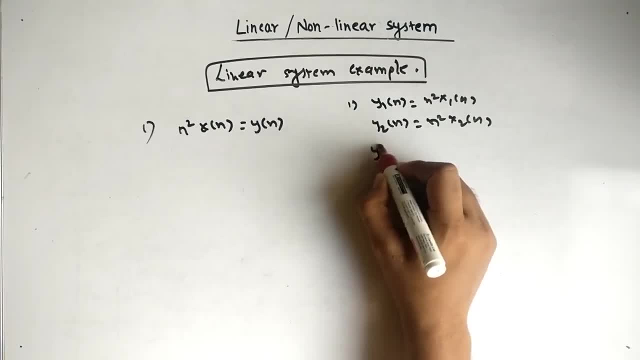 n And that is equal to discuss, for Great t was bunch xn, Again, xn family. This is crucial to get little bit of information. So the first n, then we add both this, what so we get y dash of n. adding this to will get x1 of. 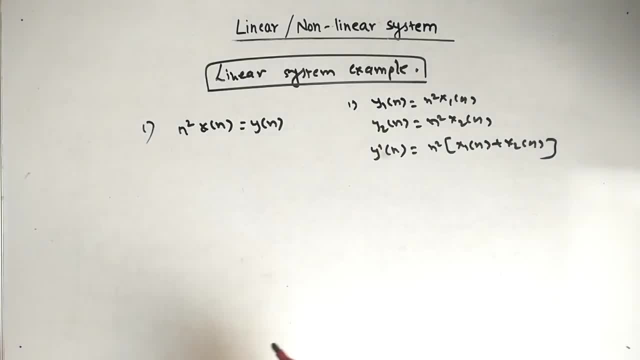 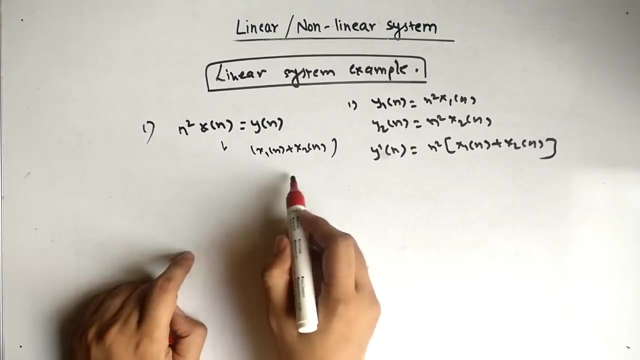 n plus x2 of n. all right now. now just imagine that we are finding y dash of y, double dash of n. y double dash of n means changing x of n to. we change this to x1 of n plus x2 of n, all right, and changing this will get the same answer. 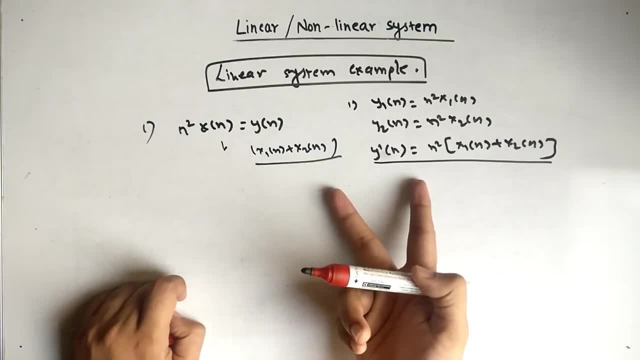 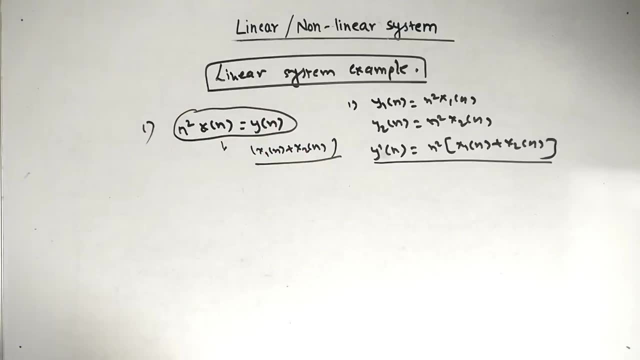 so you can see both are equal: y dash of t and y double dash of t. this means it is a linear system. so what this mean? this equation gives a very general equation. all right, so the general equation is that if we have y of, let's say, t or n, 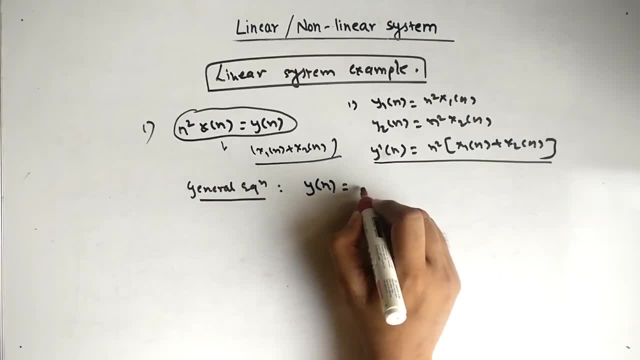 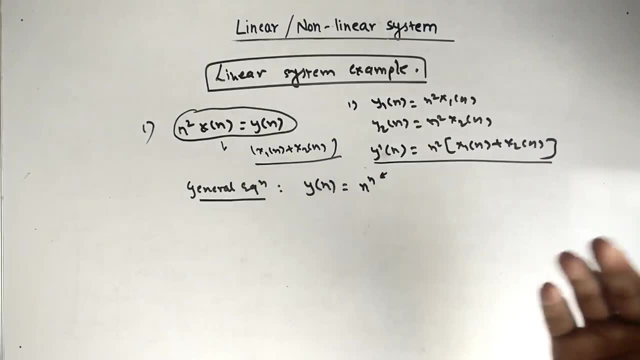 i'm taking n here. all right, the general equation is: y of n is equal to t. uh, let's say n is the variable. so n raised to n. again, n can be any value- 1, 2, 3, 4, any value- and we have x of n. if you see this, this equation, this means it is a linear. 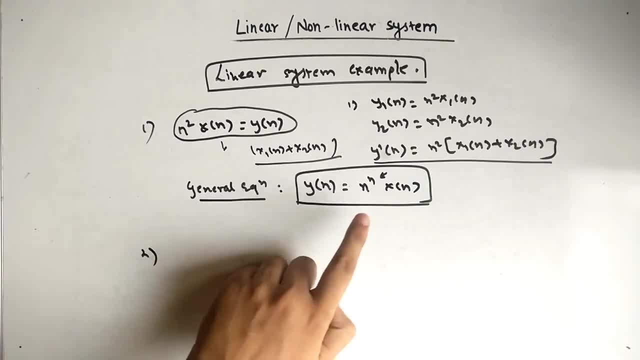 equation. all right, this was multiplying n raised to n, all right, and this small n means any value: 1, 2, 3, 4, anything. what if y of, let's say t, is equal to 10 times cos of, let's say 100 pi t and multiply by x of n? uh sorry, t is the variable, so x of t. 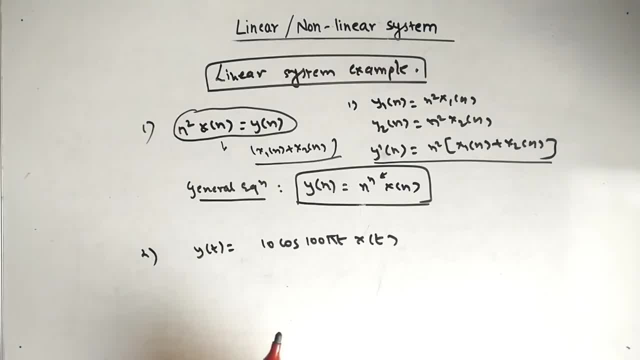 as a result of that, please repeat the same step and let's let's say, if you were to change x of t to x of t, we can add a variable for another variable, so we can't use the variable imau. we are going to do the same for the first. 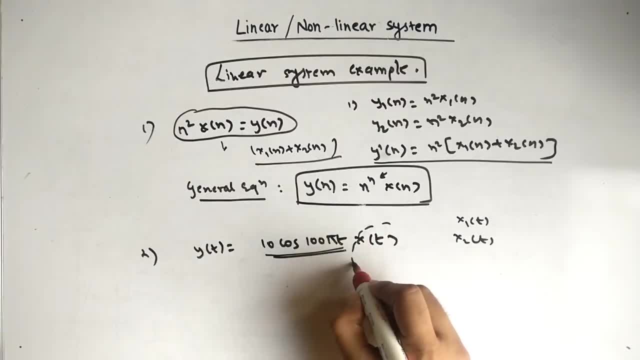 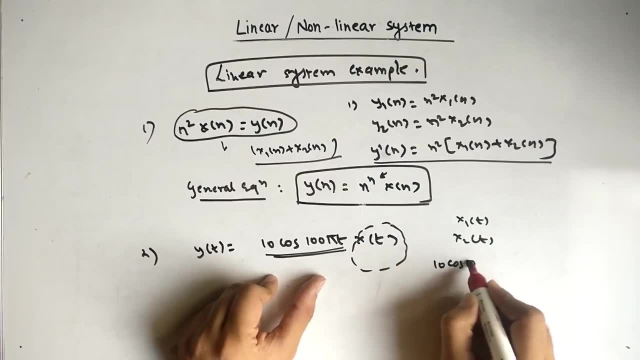 condition. now imagine that we take. now we need a constant variable. let's say we need a constant method, always with constant Sat, or i comes in same form, i comes in another form, i maintain af. what will be the answer for this? now again, you multiply this and you've got it is a linear. system. now you, when you change this, also like x1 of t and x2 of t, what changes is this? all right, then we, this remains same in both. all right, so 10 cos hundred python remain same in both. now variable changes. so when we add only these two variables, 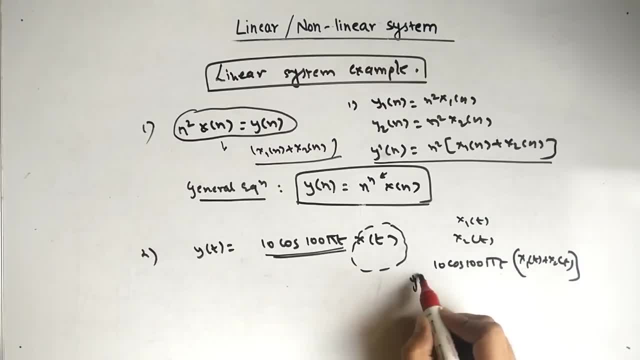 adds, all right, and we get y dash of t. fair enough, all right, let's say one more time: x1 of t will be 100, sorry, 10 cos 100 pi t. x1 of t. x2 of t will be 10 cos 100 pi t, x2 of t. then we add, then we get. 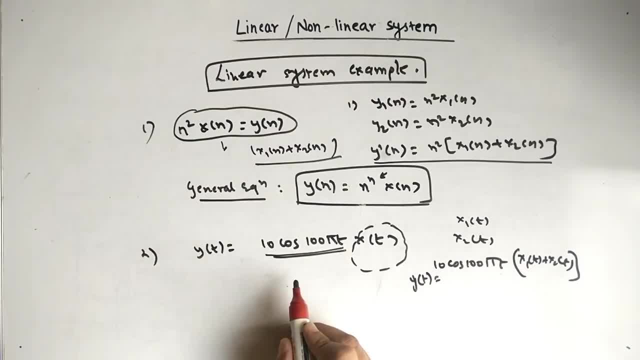 this and we get y dash of t. now talking about y double dash of t, what will happen? only this will change, and this will change to x1 of t plus x2 of t. so again both are equal. y dash of t is equal to y double dash of t. this means the system is linear system, so this can be also a general. 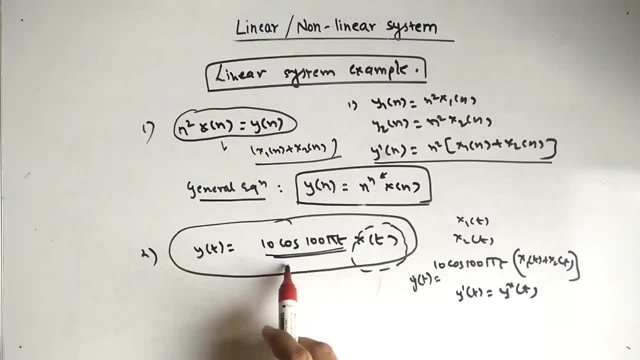 equation. all right, when we multiply anything, anything, to x of t, we get a linear system. now the important point here is: suppose i add, suppose i add, let's say anything, either n, square, or let's say 10 cos, pi, t, if i add any constant to them. let's take example t cube, and it is x of t. i have this and now i add a plus. 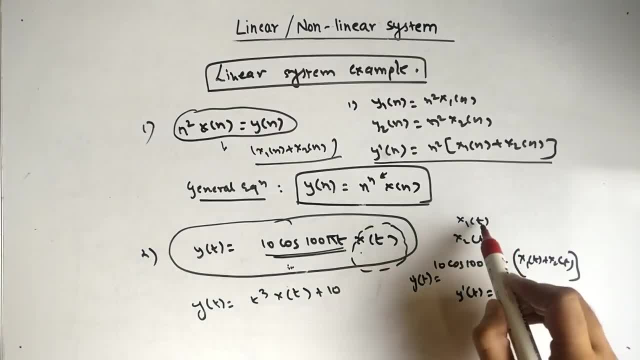 10. what will happen? what will happen is: x1 of t- we get a plus 10 here, all right. and in x2 of t, we also get all right. this will happen. we are solving this. t cube, x1 of t plus 10. t cube x2. 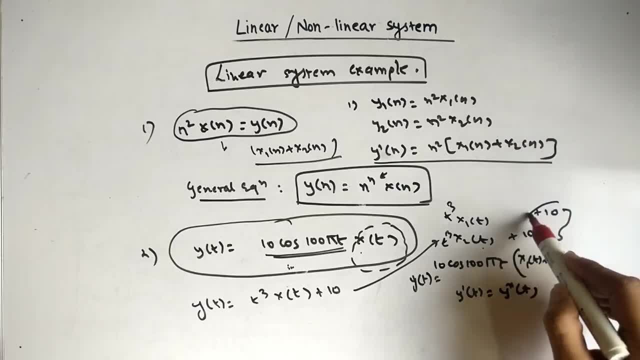 of t plus 10. now when we add both this- 10 plus 10 also added, and we give and we get 20, and 20 is in y dash of t. but when we solve for y double dash of t, what will happen? only this changes. this changes to t cube. 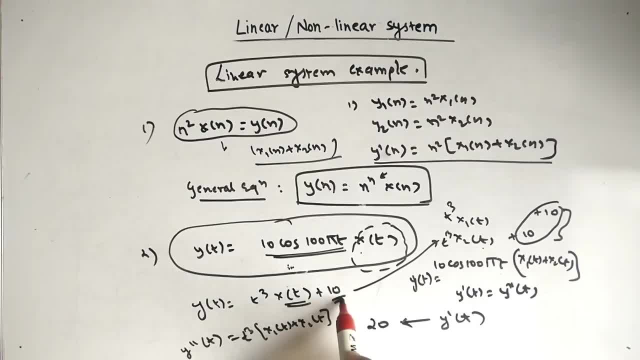 here x1 of t plus x2 of t and 10 remains. add as it is. this is not 20 here, so 10 as it is. so what is the difference? the constant changes, all right. when the constant changes both, the equation is the same. so this is a non-linear system. so remember this: this and this are linear system. 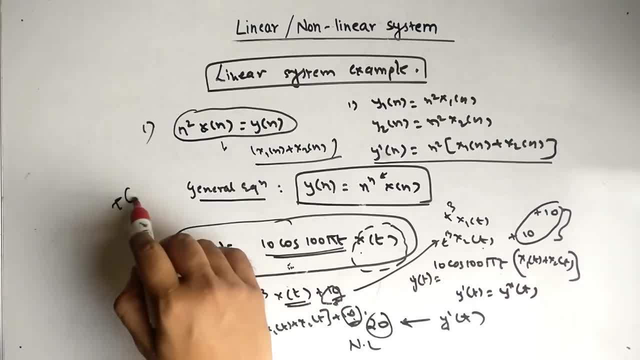 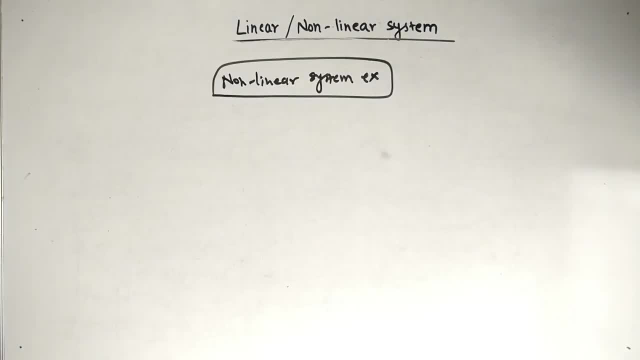 but when we add a constant, you see, when we add plus c, when we add a plus c, it becomes a non-linear system. now let's see the example of non-linear system. so first we had is we talked previously, that is, if we have y of t and let's say t raised to n, x of t, and we add a constant to it and we 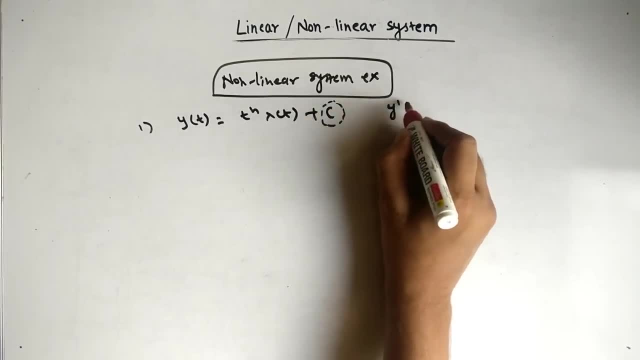 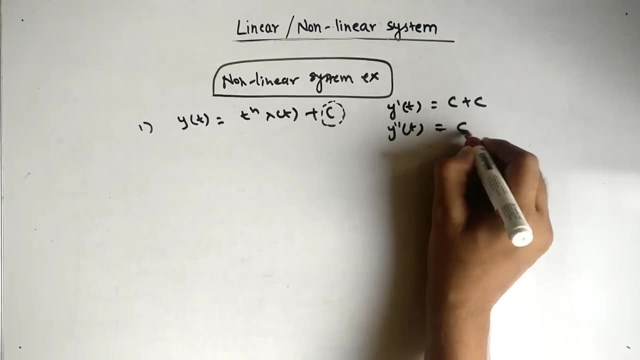 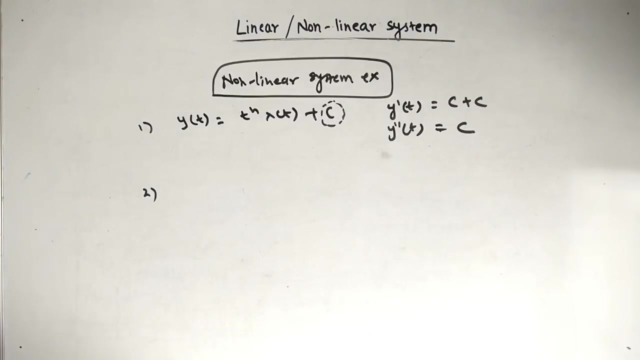 get a constant. this constant changes for y dash of t and y double dash of t. what happens is we get constant added right here, but here we have only one constant, so these two are not equal. this means it is a non-linear system. when we talk about second example, the second example is here. we 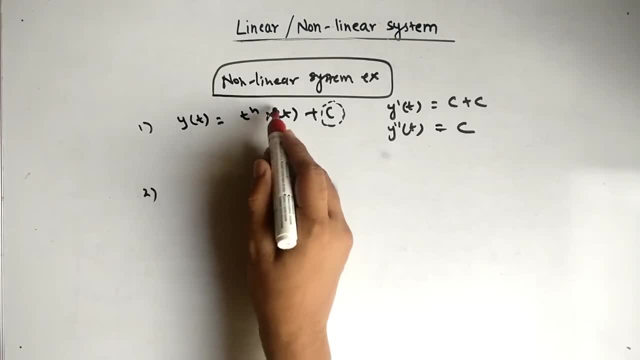 added constant in this. what about we square this? so, if we have y of t that is equal to, let's say, t into x square of t, now what will happen? let's solve this. so first step is finding y dash of t. all right, for this we need two y, one of t, and 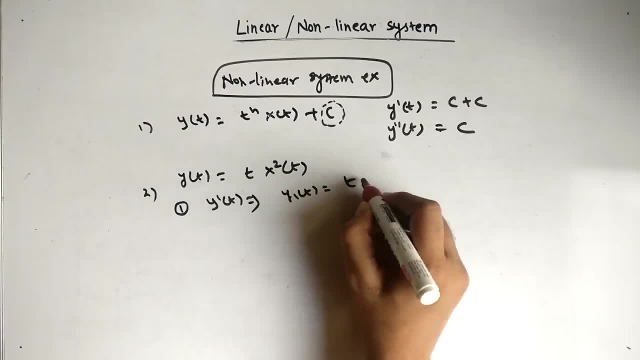 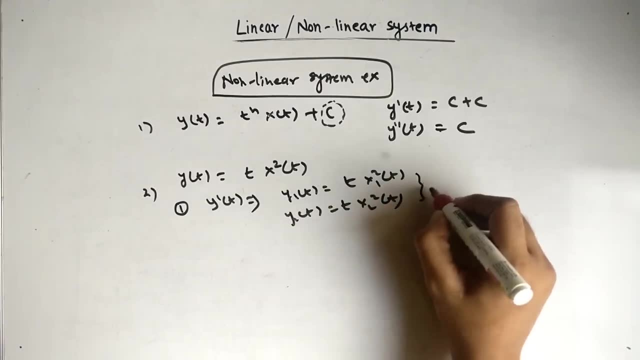 y, y two of t. so y one of t is t times x one square of t, and y two of t is t times x, two square of t. all right now, adding this two, we get t common, but x one of square. this two get added, so x one square. 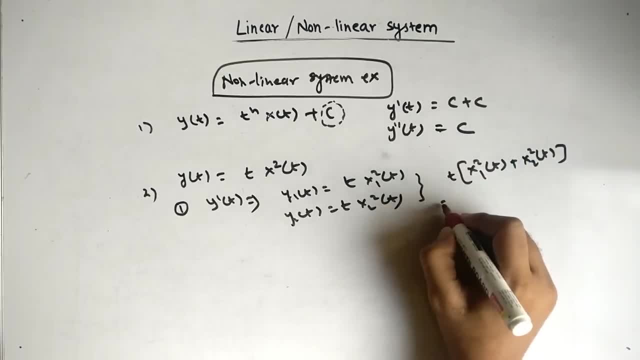 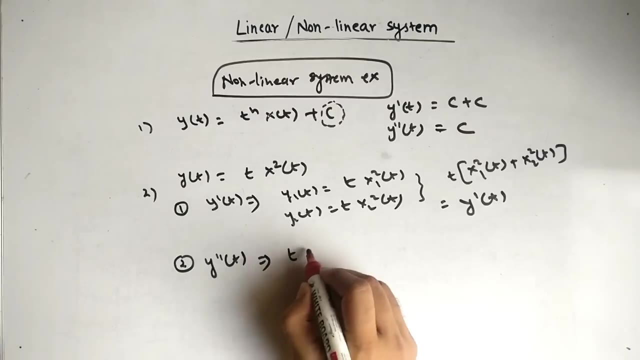 of t plus x two square of t. so this is nothing but y dash of t. all right, now we have y dash of t finding y double dash of t. for y double dash of t, we need x of t, change to x one of t plus x two of t. so what will happen? right here? 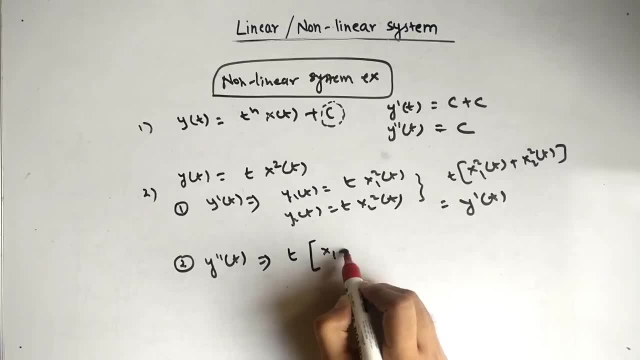 this is important. see: x one plus x two. all right, let me write this way: x one of t plus x two of t, and it will become the whole square. all right, now you can see. now you can see the difference. so this is the whole square. why see closely? we have x of t, the. 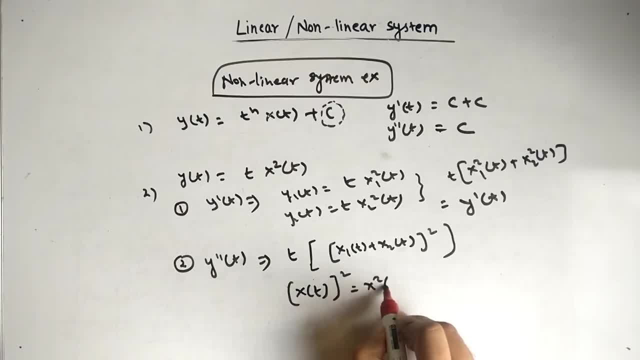 whole square. this means this: and this are equal: x square of t. all right, now we are replacing x of t to x, one of t plus x, two of t. that's why we get this all right, and you can see this- and this are not equal. so again, this equation is very important, so this gets added to a non-linear. 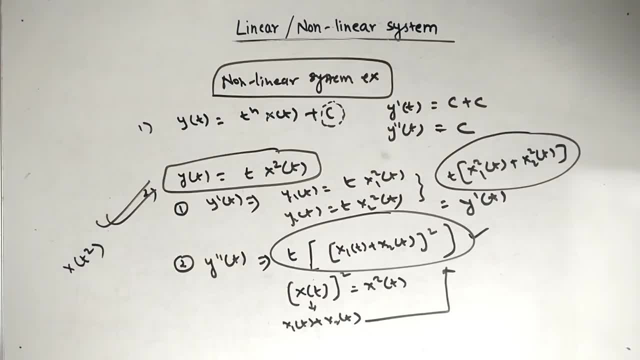 system. what if i had x of t square and not x square of t? then this is linear. now why it is linear? solve it. when you solve it, we get x 1 of t square, x 1 of t square, then we get x 2 of t square. 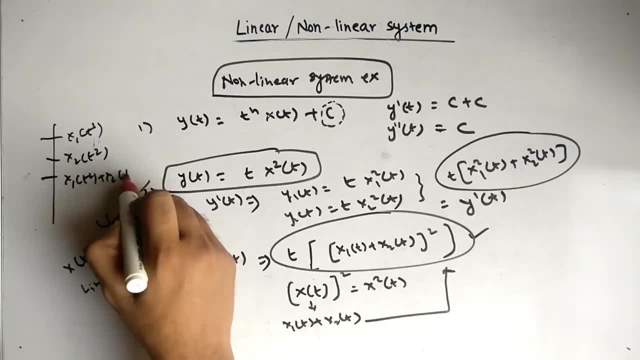 then we add: then we get x 1 of t square plus x2 of t square. now, when we change this- now let's see closely- we have this all right. we are changing only this x1 of something. let's say, right, this way: x1 of something plus x2 of something. so this: 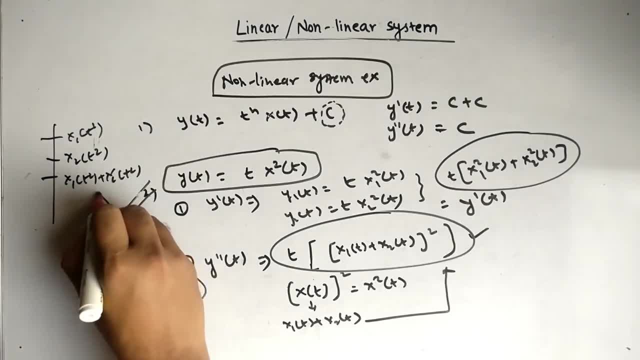 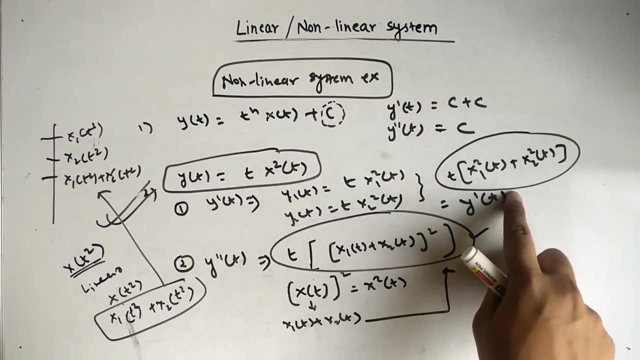 won't change this and this will remain same. so y dash of t and y double dash of t remain same, but here, when we replace x of t, we get x1 of t plus x2 of t, the whole square. you can see the whole square and here the equation equation is different. that's why this is very important example and 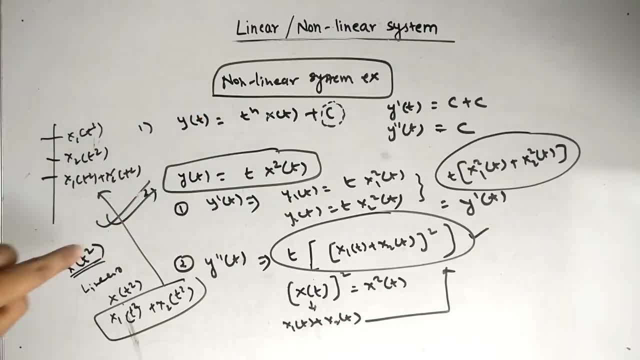 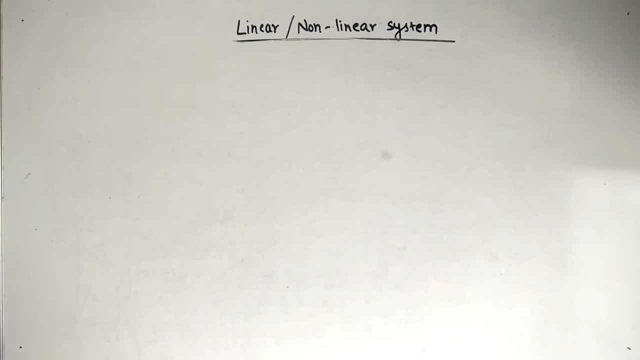 don't get, don't get confused between x square of t and x of t square. now let's take the last, very important equation, and the equation is: y of t is equal to e raised to x of t. so let's solve this. first, x1 of t has input. then we get y1 of t, that is equal to e raised to x1 of t. 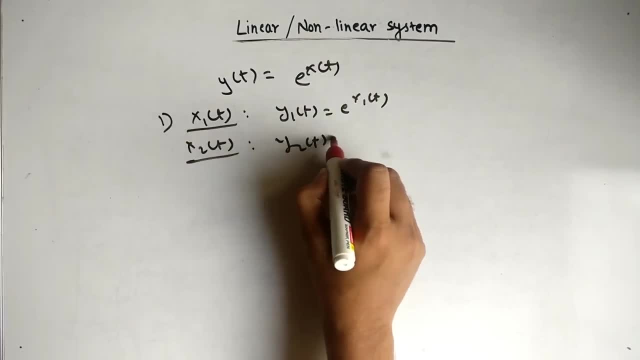 all right, then we have x2 of t, and y2 of t is equal to e raised to x2 of t. all right, now we have to find y dash of t that is equal to e raised to x1 of t, plus e raised to x2 of t. fair enough, 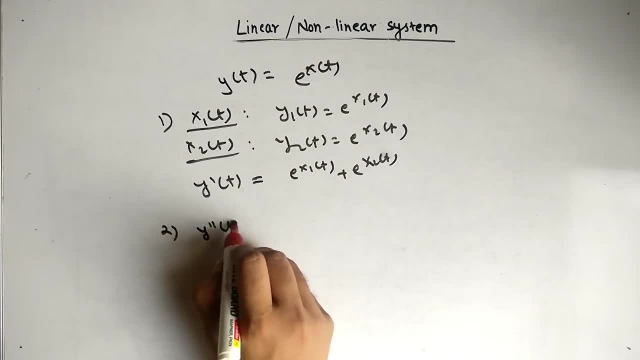 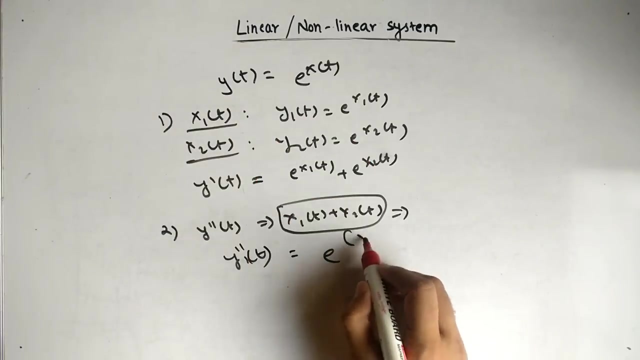 all, right now we have to find y double dash of t. for that we have input x1 of t plus x2 of t as our input. so what is y double dash of t? this will be e raised to replacing this. it would be x1 of t plus x2 of t. 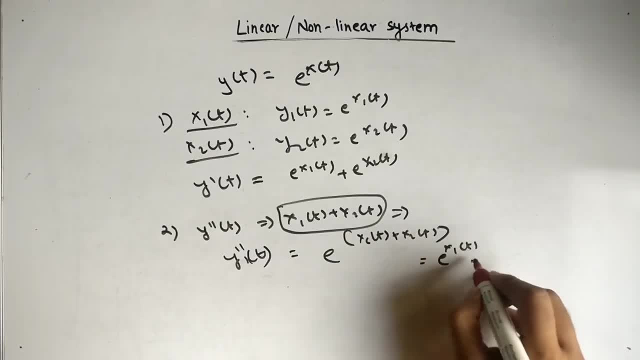 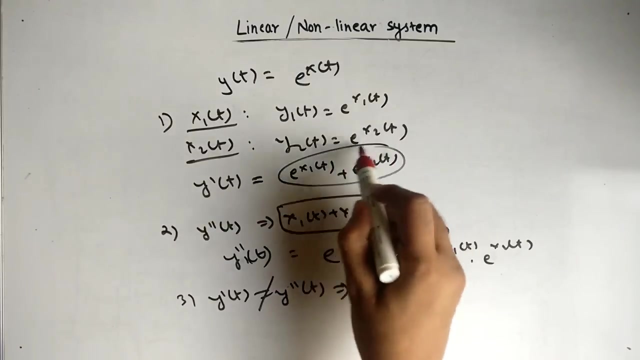 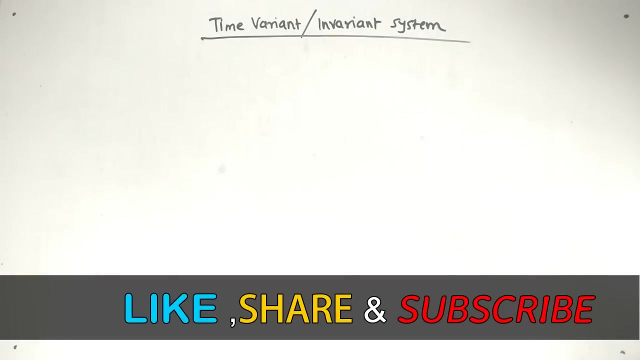 now this means e raised to x1 of t into e raised to x2 of t. all right, and now you can see y dash of t is not equal to y double dash of t. this means system is non-linear system. you can see this that way. hello friends. today we will see the very important topic, and the topic is time variant and 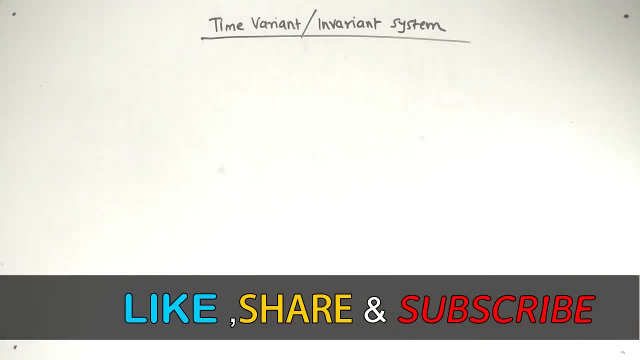 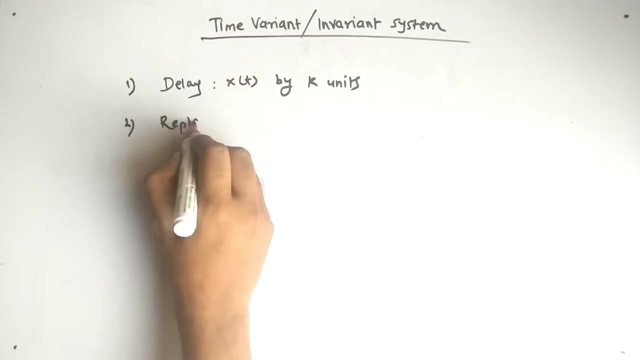 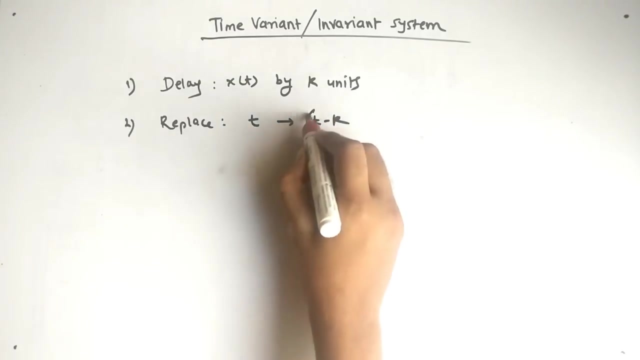 invariant system. so let's see first how to find out whether a system is a time variant or invariant. we have to follow only two step. first, we have to delay, delay x of t by k, by k units, okay. and second, you have to replace, wherever you see T, replace it by T minus K, now, if one equal to if delay. and 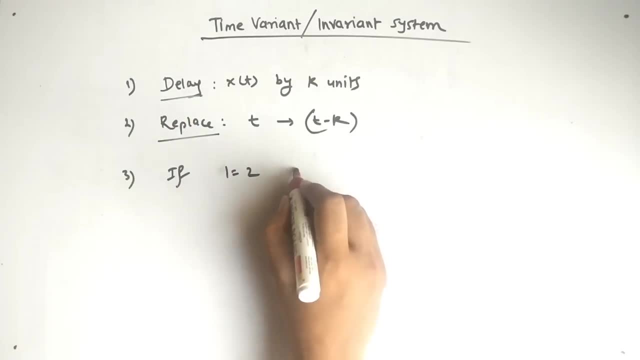 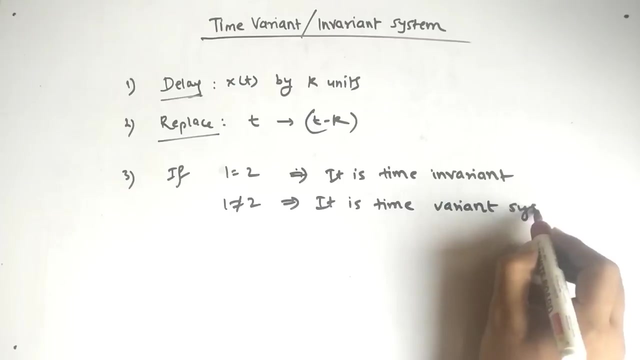 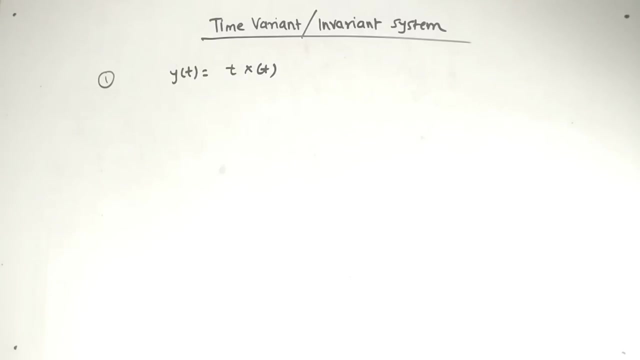 replace. both are equal, then. or let's say: then it is time invariant system. if one is not equal to two, that means it depends, that is, it is time variant, time variant system. only you have to follow these two steps: delay and replace. so let's see the examples on this. so our first example is: Y of T equal to T into 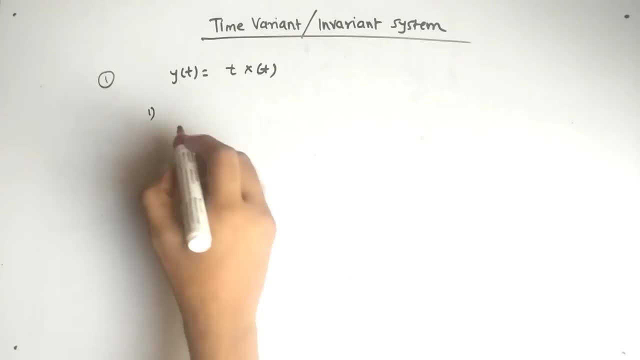 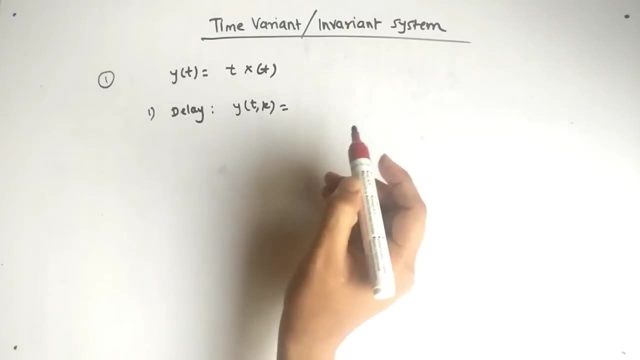 X of T. okay, so our first step was to delay. let delay be represented by Y of T comma K. so we have to delay what X of T? so T will remain as it is and X of T is delayed. it is delayed by K units. okay. now, second step is replace, replace. wherever you see T, replace it by T minus. 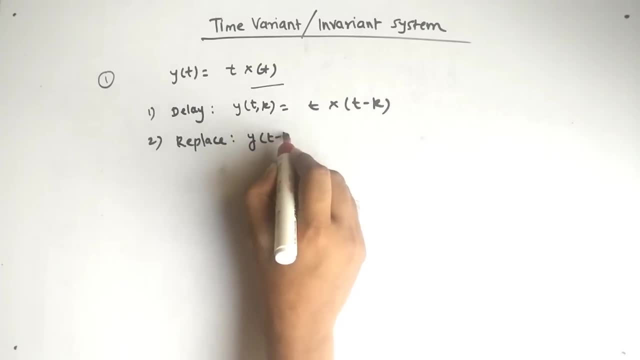 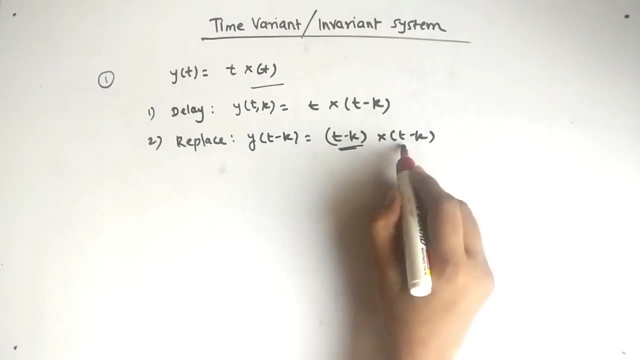 K. so let replace be represented as T minus K. and now T will be changed to T minus K, X of T minus K again. so you can see it is replaced by T minus K. now. third step was was to check whether one equal to or one is not equal to two. so you can see that one is not equal to two. you can. 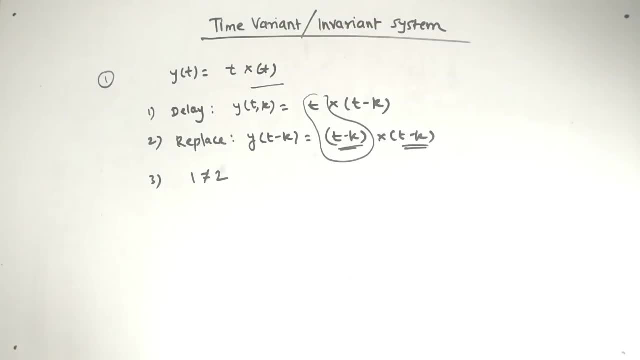 see, these terms are different, so one is not equal to two. so what does it mean? it means that it is time. variant system. I hope it is clear to you. so now let's solve orally all this question. so our first question is X of T minus 3 U of T. so I have already told that X of T will be delayed. all right, so 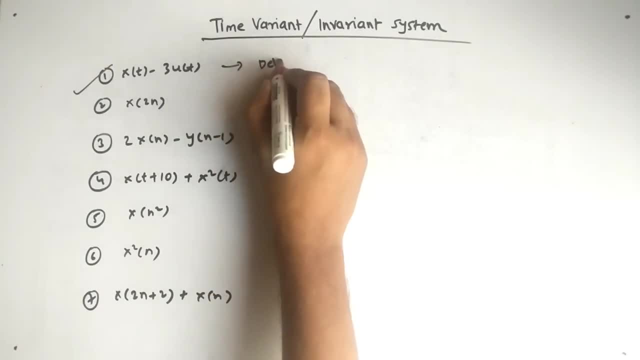 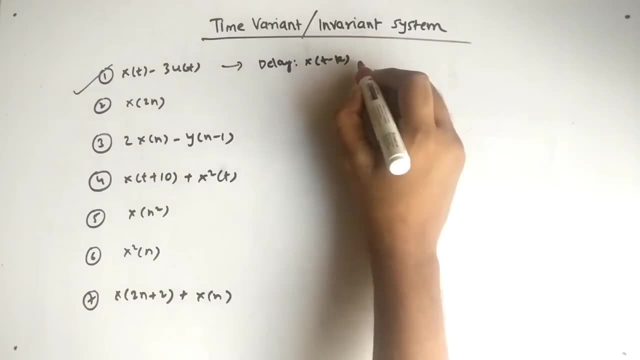 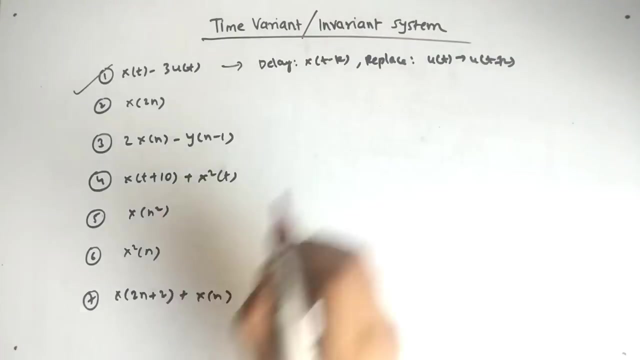 U of T is unchanged. so in delay X of T minus K happens, but U of T remains same. but when you, 3 remains same. but when we replace U, of T also changes to U of T minus K. so clearly, 1 is 0 equal to 2. this means it is time variant. alright, so let's take another example. 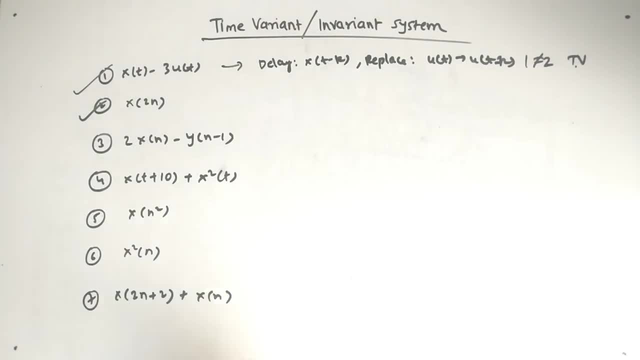 second example is X of 2N, now X of 2N, again in delay. what will happen? X of 2N minus K, but in replace it will be x of 2 times n minus k. so again, both are not equal. so it is time. 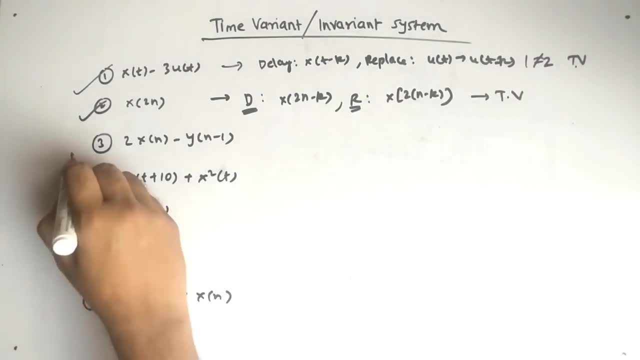 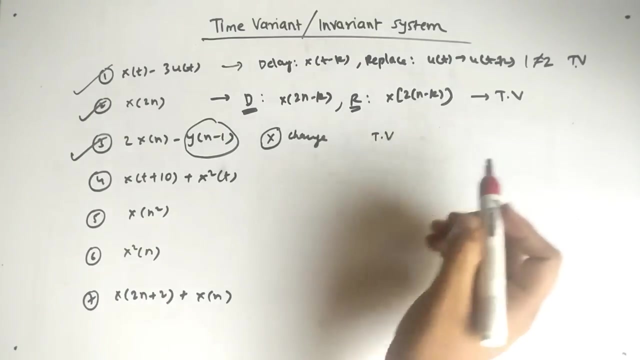 variant. now taking third example: what does third example says again, it has y of n minus k. it will not change in delay. when will delay? only x changes. x will change when y is unchanged. therefore, but in replace y will change. therefore, it is time variant. why? because 1 is not equal to 2. now taking 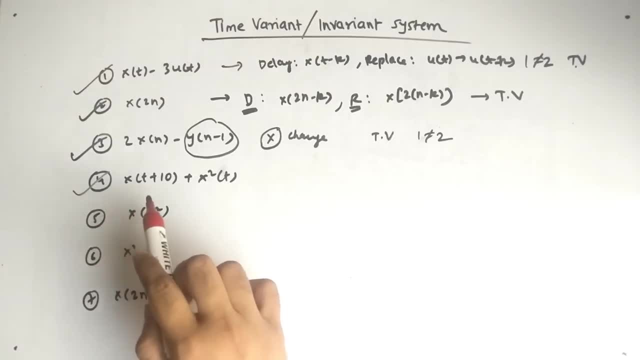 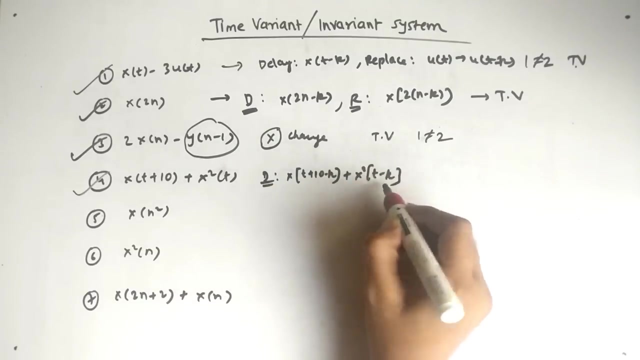 the fourth example. fourth example is very interesting. like, say, x of t plus 10 plus x square t, now in delay. it is simple: like t plus 10 minus k and again plus x square t minus k, and when we replace it again we get the same terms like t. if we replace, we get t minus k, and again we replace t, then we get t plus 10. 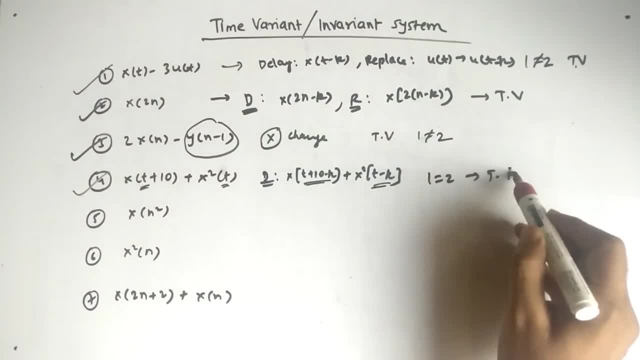 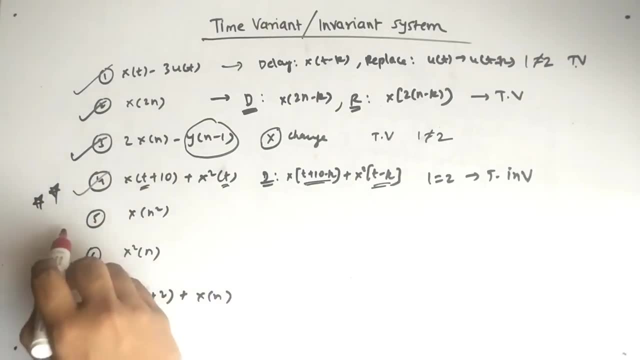 minus k, so 1 is equal to 2. this means it is time invariant. this was important. you can mark it as important. now, taking the fifth example, these two example are very interesting because this will create a dengan all your concepts: x of n square. now what a? what does this mean? X of n square, when we delay x. 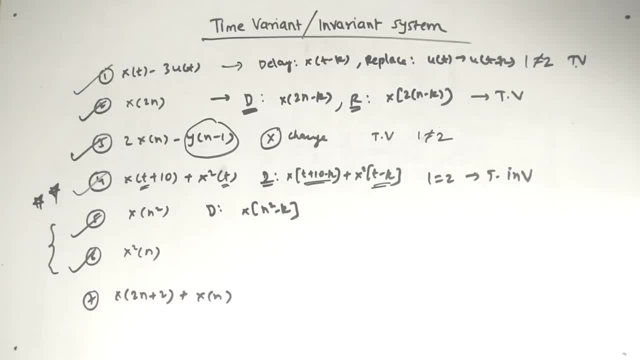 of n square minus k will happen, because it is not x square n, it is x of n square. so in delay this will happen, but in replace it will be n minus k, the whole square. so 1 is not equal to 2. this means it is time variant. okay, now come the x square n part. 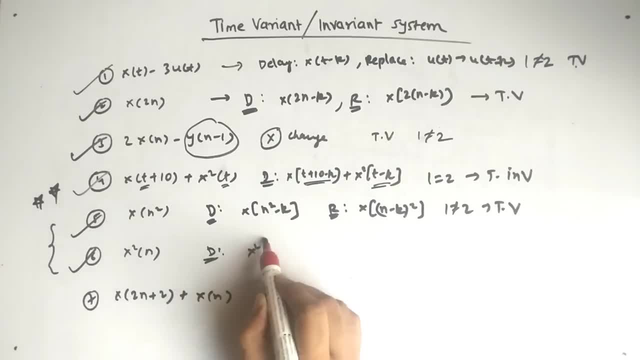 x square n part is simple, like: when we delay, it is n minus k and again when we replace, it is n minus k. So 1 is equal to 2. this is time invariant system. So this was also very interesting. So note 4, 5, 6, because it is very important. functions Now. taking the 7th, 7th: 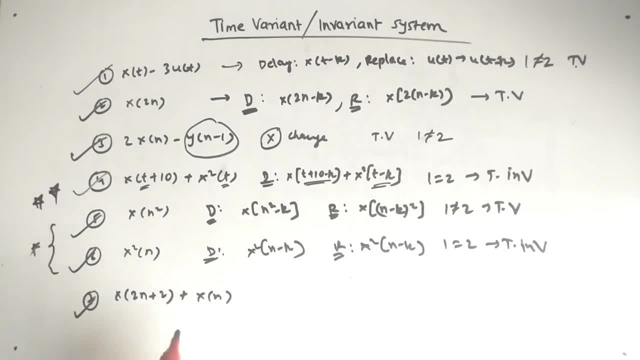 is x of 2n plus 2 plus x of n. Now, when we delay, Delay means this function will be delayed: 2n plus 2 minus k. But when we replace this, n will be replaced, So n minus k plus 2.. Again. 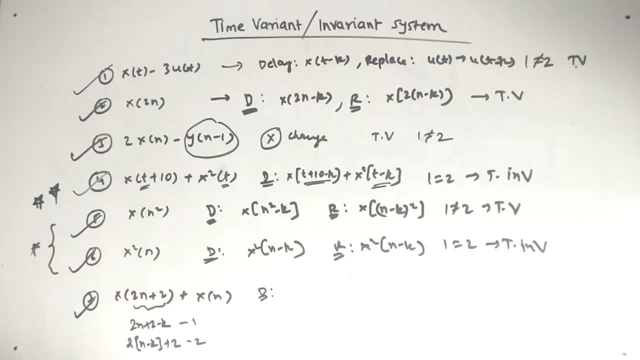 these two are not same. This is 1, this is 2.. These are not same. So when we delay, x of 2n plus 2 minus k is the different part, and when we replace x of 2n plus 2 minus k, 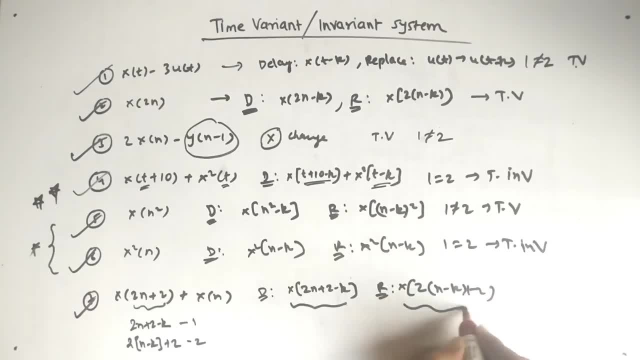 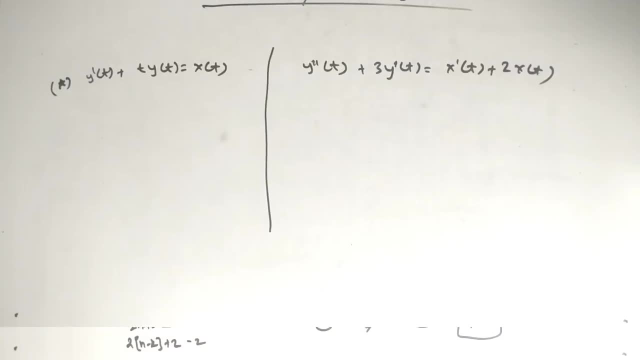 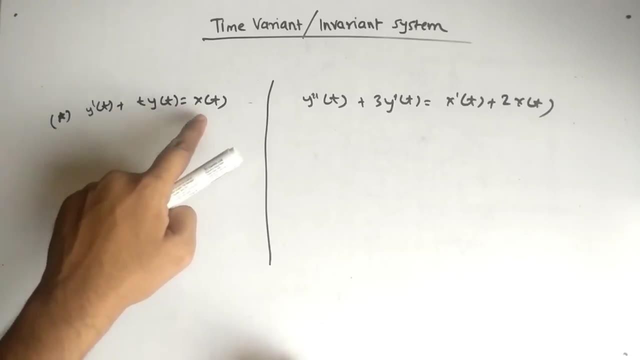 2 times n minus k plus 2.. This is different, So 1 is not equal to 2.. Therefore it is time variant. Now let's see these two equations like: y dash of t plus t times y of t, equal to x of t. and the second question is: y double dash of t plus 3 times y dash of t, equal to. 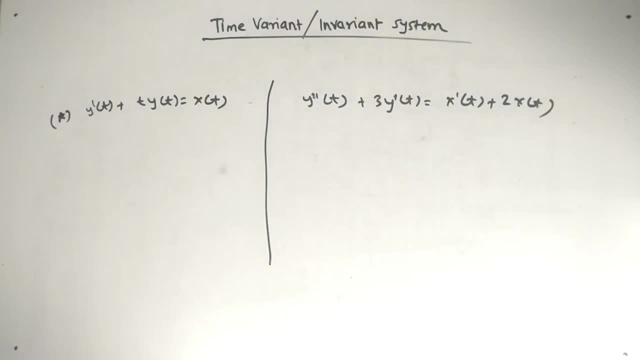 x, dash of t plus 2 times x of t. What is different between these two equations? This part, This part Here in this t term is multiplied by any of the function, like y of t or x of t. T term is multiplied, But in this there is no t term. So simple: If t term is multiplied, this means 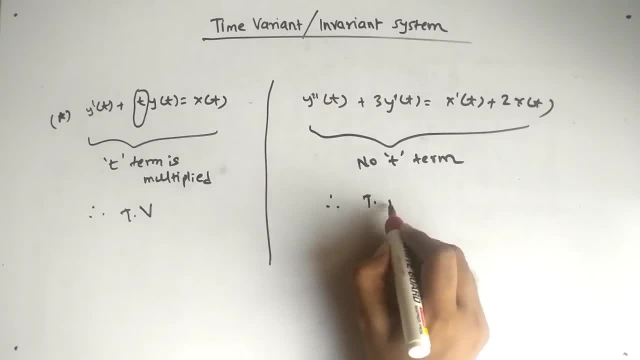 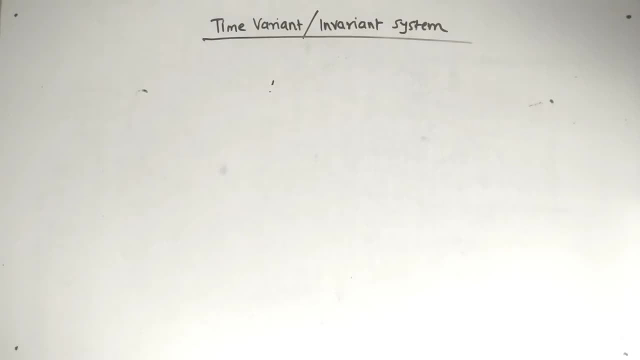 it is time variant. There is no t. this is time invariant. Ok, Again, there is one important equation, that is x of minus t. When we see this x of minus t, you delay it. When we delay it, x of minus t changes to x of minus t minus k. We delayed. 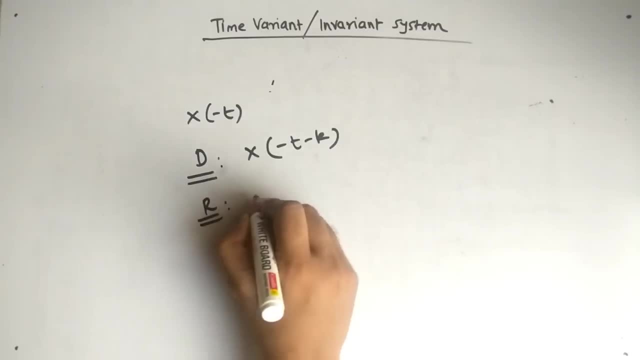 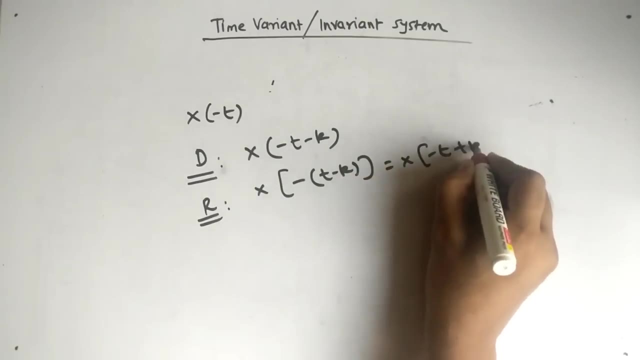 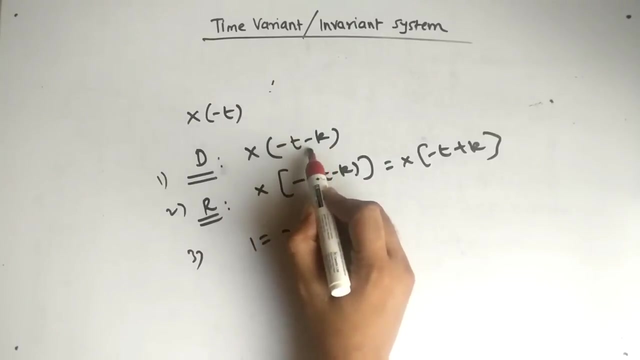 it by minus k unit. But when we replace then it becomes minus of t minus k. That is equal to x of minus t minus k. So this is x of minus t minus k. So this is x of minus t minus k, plus k. so one, two. so third step: was one, two, equal or not? you can see minus k and plus k. 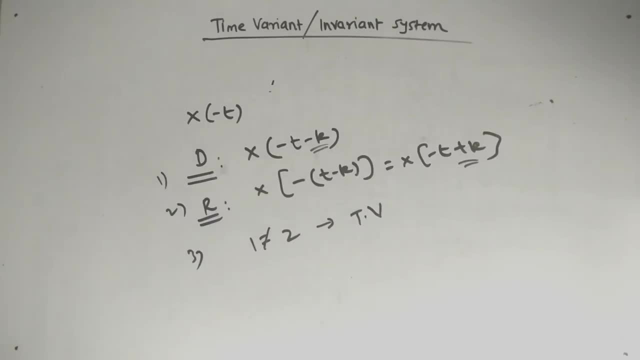 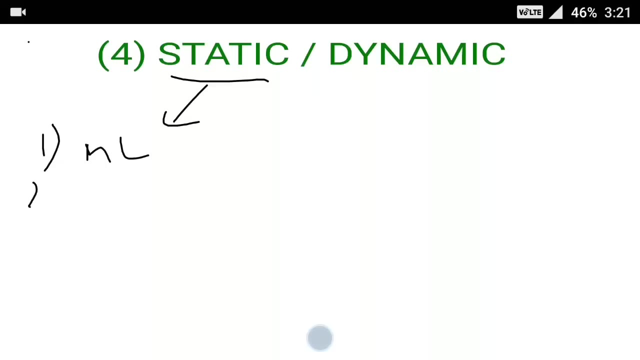 so it is not equal. this means it is a time variant system. so is ko hum bolte hai memory less system. first point ye hai. second point ye hai ke isme time shift jo hai woh nahi hota. toh, agar dynamic system ki baat kare, toh uska hi opposite hai, isko memory system bolte hai. 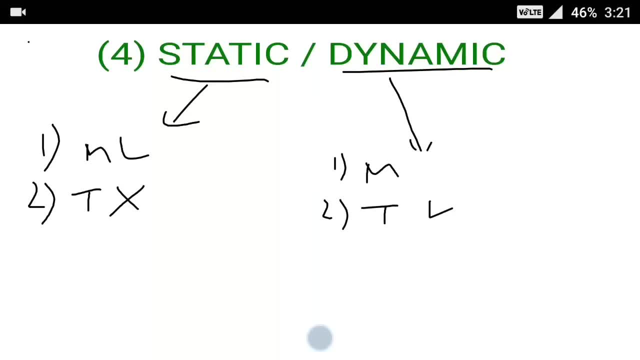 aur yaha pe jo time shift hai, woh possible hai. ab identify karna easy hai. dynamic ko kyunke yaha pe jo hota hai. integral sign: apko jaha pe bhi dikha, toh woh dynamic hai. derivative sign: dikha, toh bhi dynamic hai. aur delay sign. and last is summation sign.